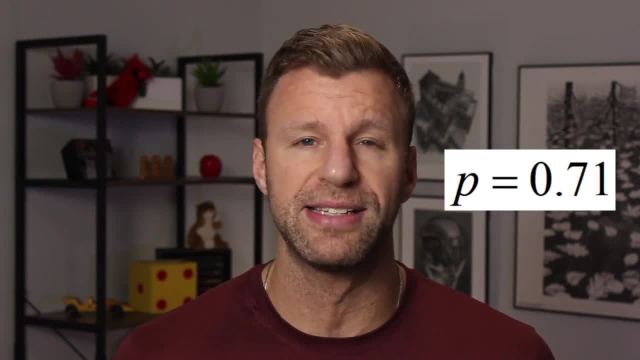 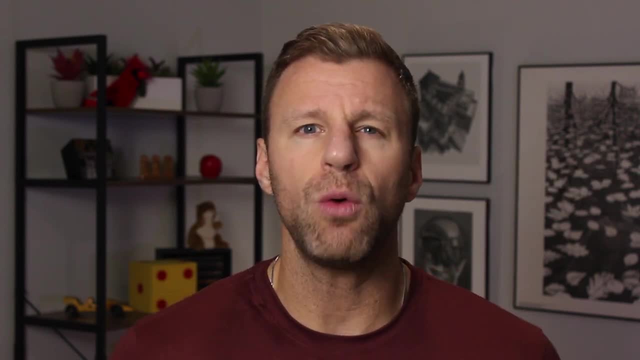 differentiate between the true p that we know. that's true for the entire United States, that's the 71 percent, and our sample proportion. that's just true. well, for our sample, 230 students. Now, what do we expect our sample proportion to be? We haven't even selected the 230 kids yet. we're 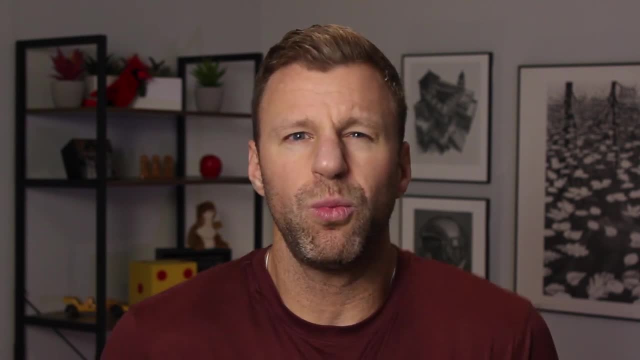 getting ready to. we're going to ask them if they believe in the tooth fairy and, you know, I guess we would expect to get something around 71 percent, because that's what's true. But samples do one thing very, very well, and that is that they. 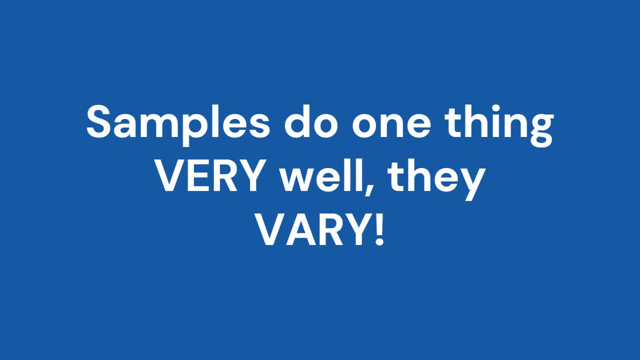 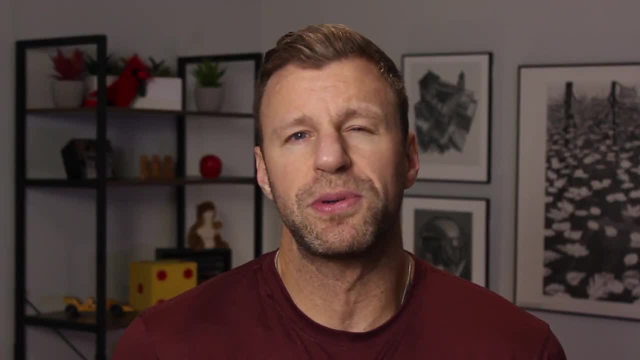 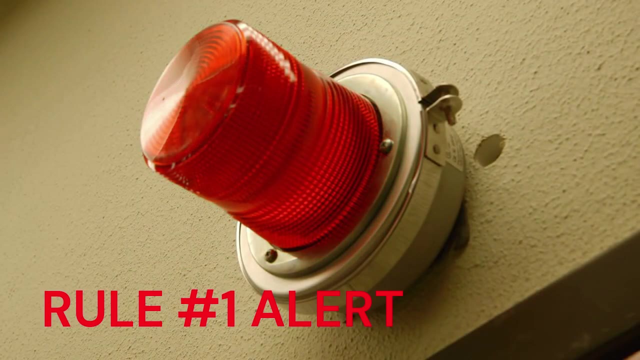 vary. See what I did there: vary v-e-r-y, v-a-r-y. okay, yeah, you get it. but that's the idea is that samples vary, and just because we expect to get 71 percent doesn't mean that we will. Now, before we go any further, we got to talk about one out of three really important rules, and that is that it 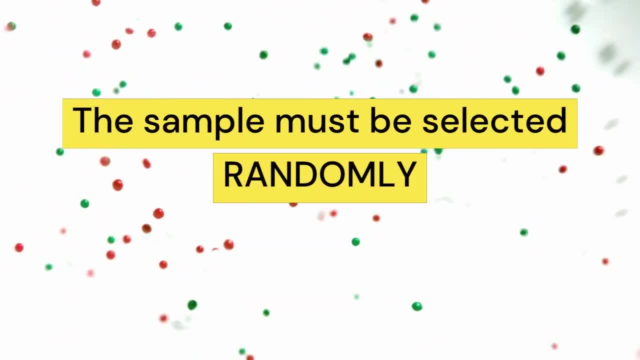 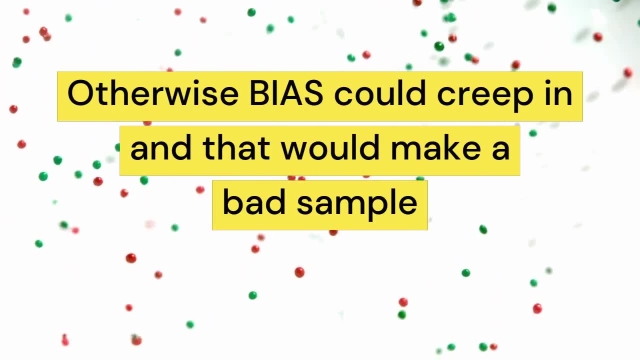 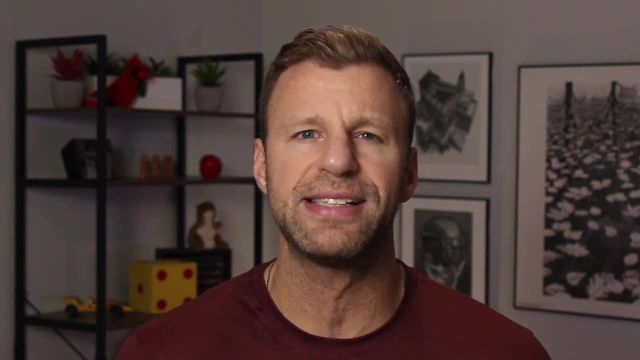 does have to be a random sample, because if it's not random then we allow a little bit of bias to possibly creep into our sample. and if we have bias in our sample we might get a little bit of bias. We might not get what we want. for example, if we just had a pure convenience, ask 230 kids at one. 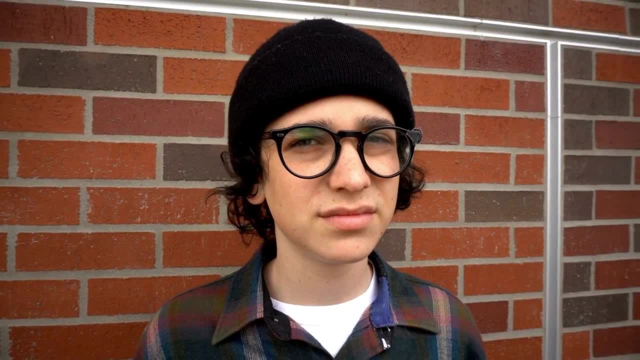 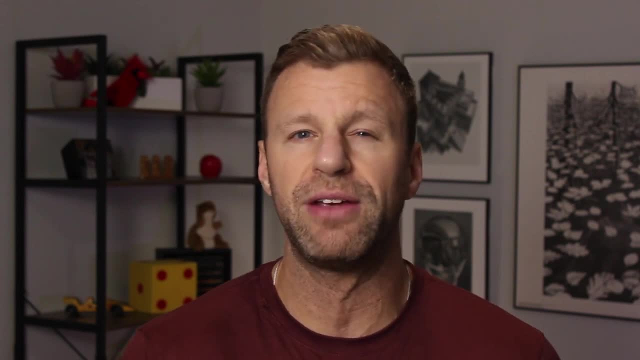 elementary school. well, there could be that one student, Billy, who's already gone around the entire school and told everybody that the tooth fairy doesn't exist. so from that sample we're probably going to get a very, very, very low proportion of kids that believe the tooth fairy, and it's not. 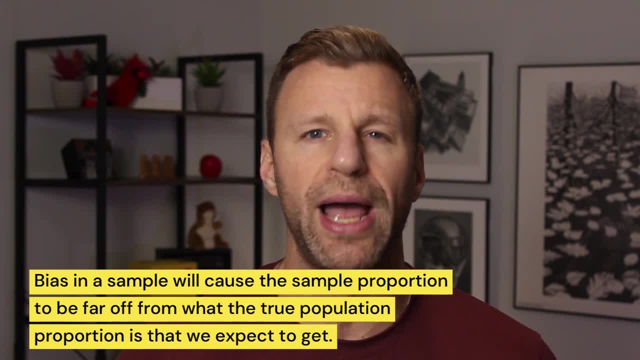 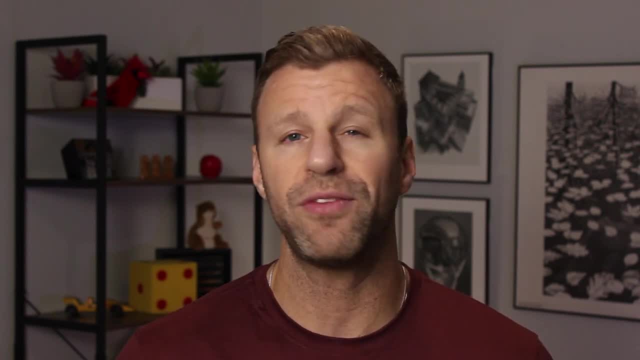 going to be anywhere near the 71 percent. that's true. So samples do have to vary and they do have to be random, and if they're not random, you have bias. and if you have bias, then you're going to have bias. Well, everything I'm teaching this video is not going to be correct. Now, the truth is. 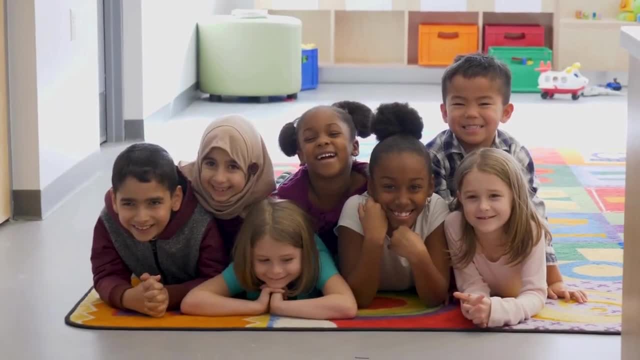 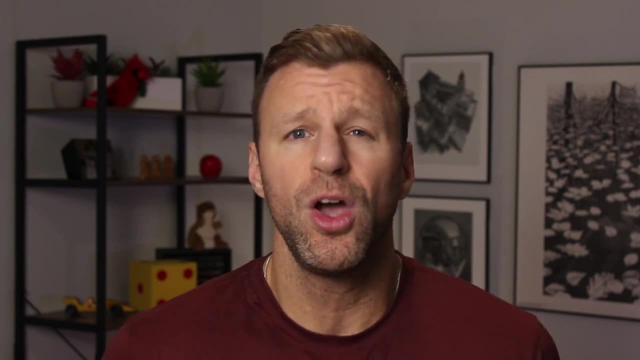 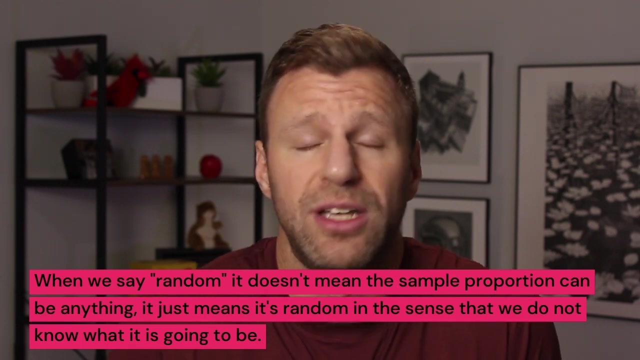 before we even take a look at that sample of 230 kids, we truly have no idea what that sample proportion is going to be. It's well random. We do know that it's going to be a number between zero and one, but we don't know exactly what's going to be. Certainly we would expect 71 percent, but again, 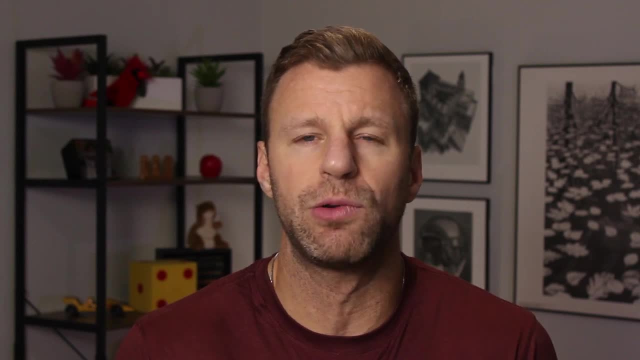 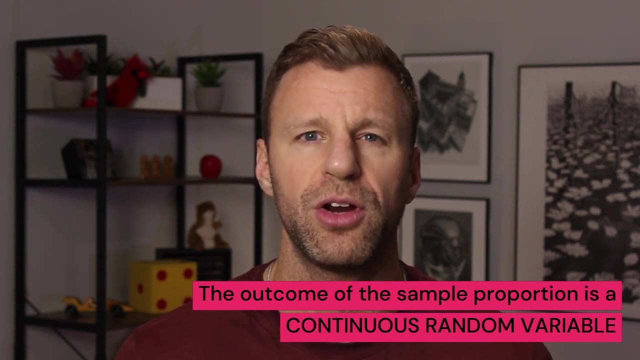 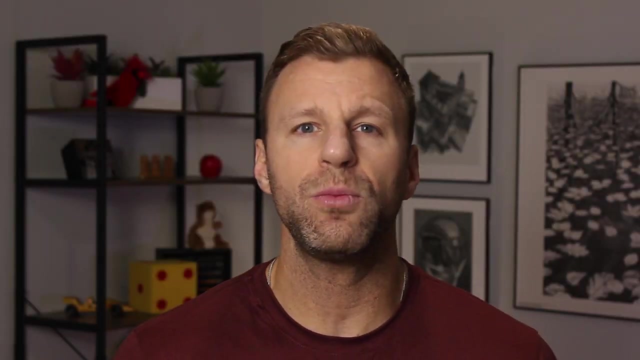 samples vary, so it might not be exactly 71 percent. So what this means is that we could actually view the sample proportion as a continuous random variable. All right, so maybe after all the dust settles and we ask all the kids in our sample, do you believe in the tooth fairy? and we come back with a sample proportion of 65 percent. Okay, a. 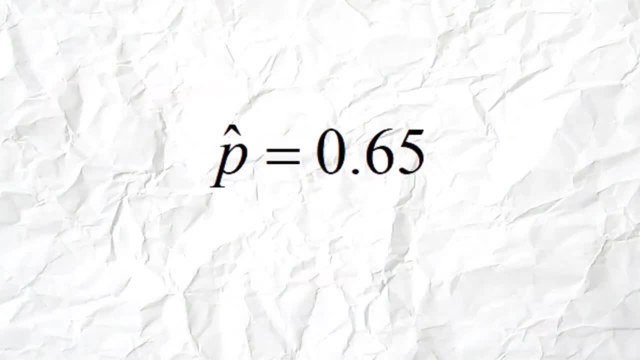 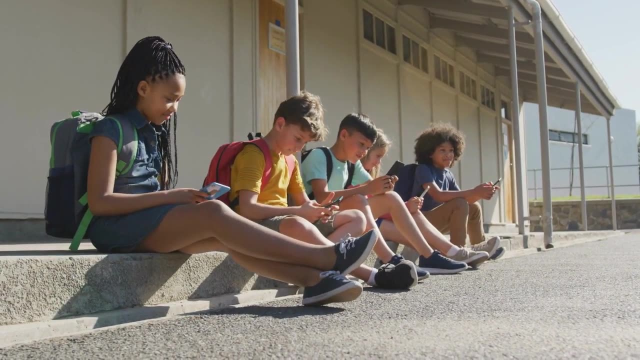 little bit lower than 71 percent and no big deal. Now what if we decide to go ahead and get a whole another sample of 230 random 10-year-olds from across the United States? What would we expect that sample to be? Well, we would expect it to be nine percent and we would expect it to be: 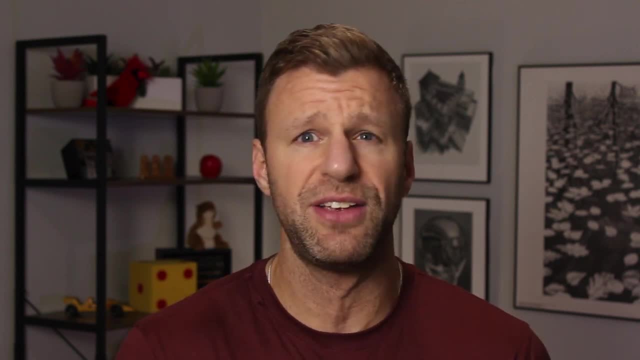 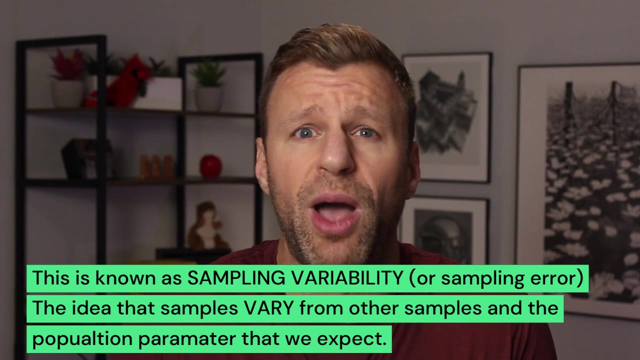 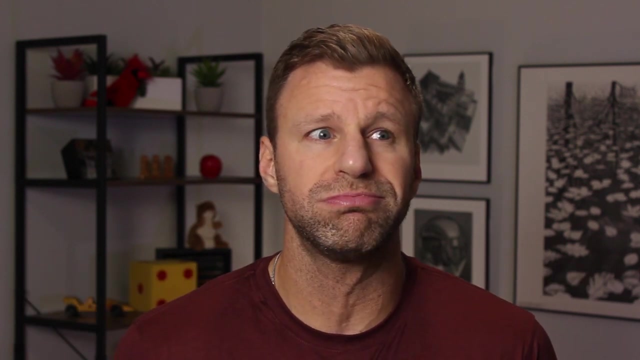 near 71 percent, but it's not guaranteed to be 65 percent either, because that's just what our other samples showed. So the next sample is going to be well its own thing as well, because, again, the sample proportion is a continuous random variable. That means the outcome could be a number well whatever. 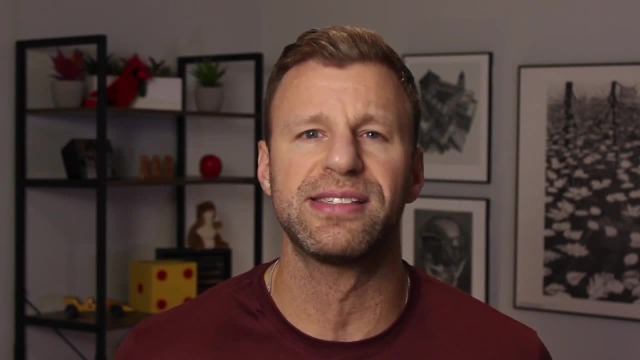 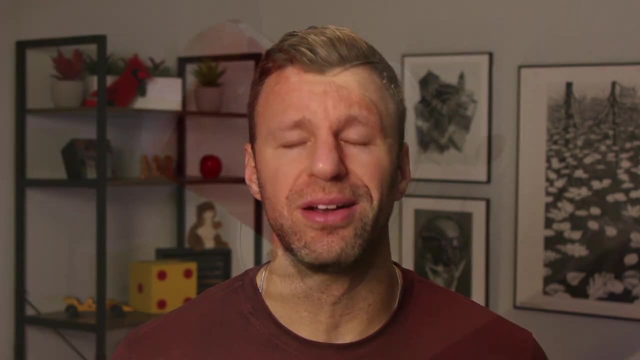 number it ends up being: Maybe we get 72 percent in that second sample that said: yes, they believe in the tooth fairy. Now here comes rule number two out of three that we got to talk about. Since we're talking about not just one sample, but a second sample, maybe even a third sample we need. 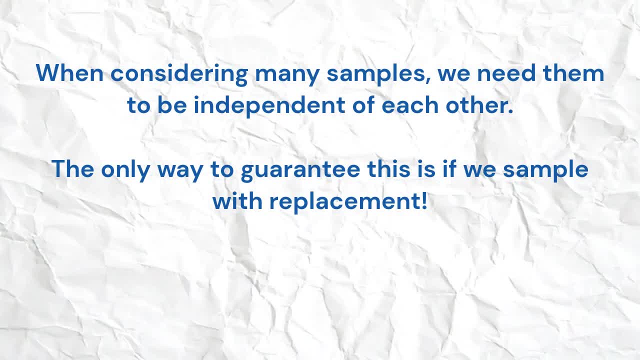 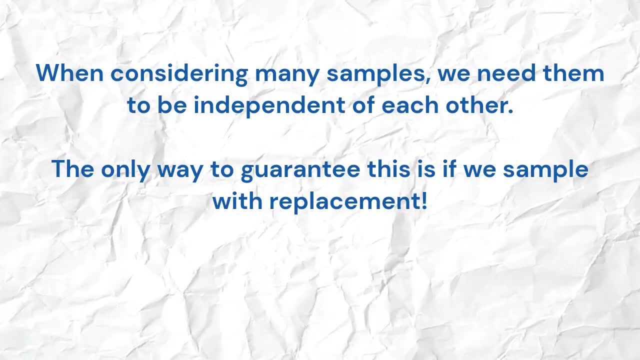 these samples to be independent of each other. and the only way to guarantee that my second sample is independent from the first sample is if, after I take that first sample of kids, I put them all back to possibly be picked again. But in the real world we typically don't do that. When we sample, we don't. 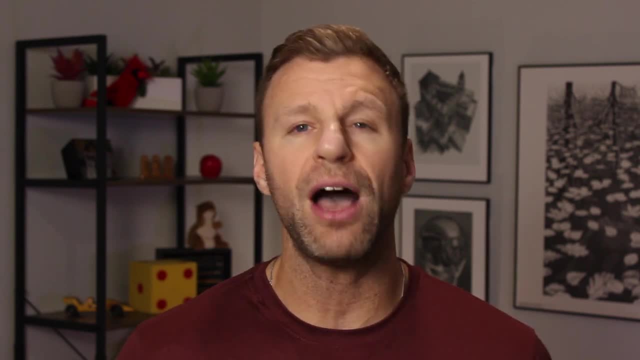 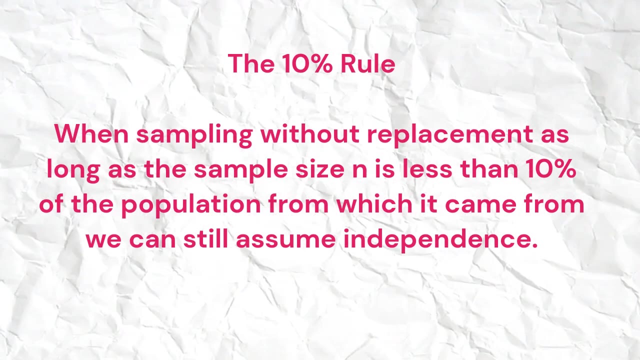 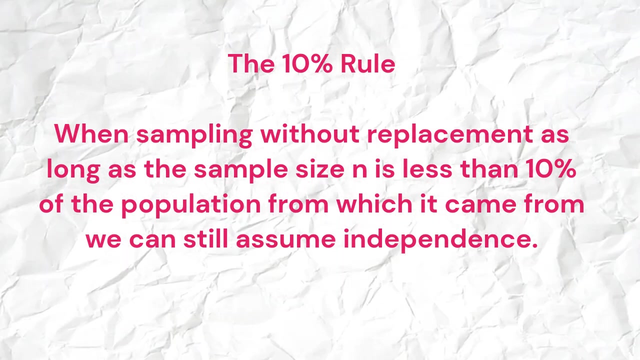 think about putting the first sample or the second sample back. Now we actually have a rule that says in our case, 230 is less than 10 percent of the entire population from which we were picking from. then we can still assume independence, even if we don't put that sample back Now technically, because 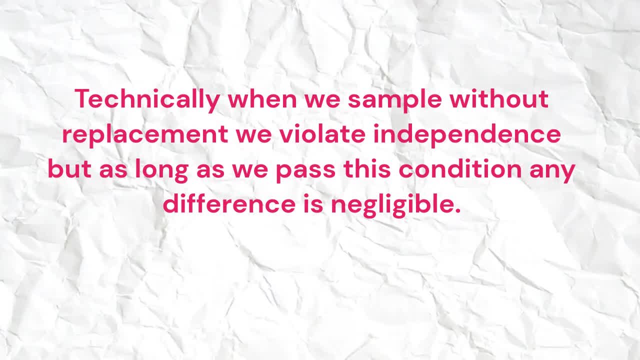 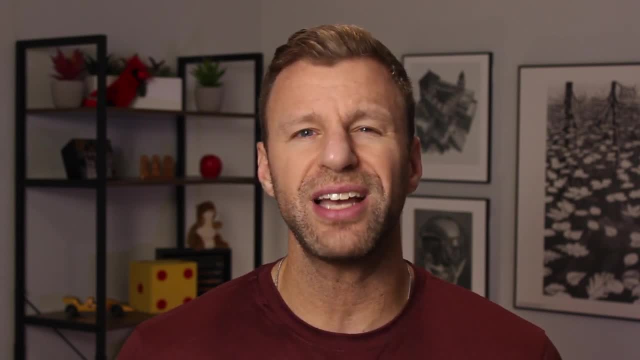 we're not putting that sample back, we are violating independence. but any difference is negligible as long as our sample size is under 10 percent of the population. So selecting 230 kids, I would assume, is under 10 percent of the millions of 10 year old kids that are living in the United States. 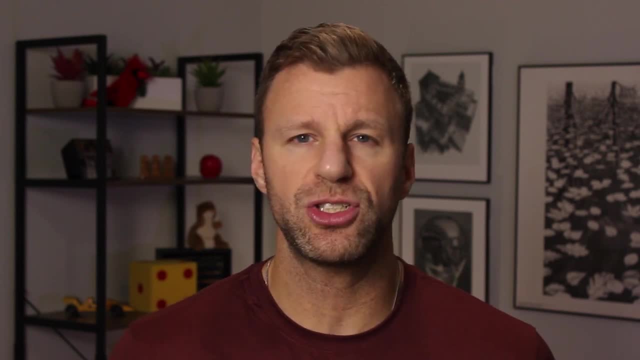 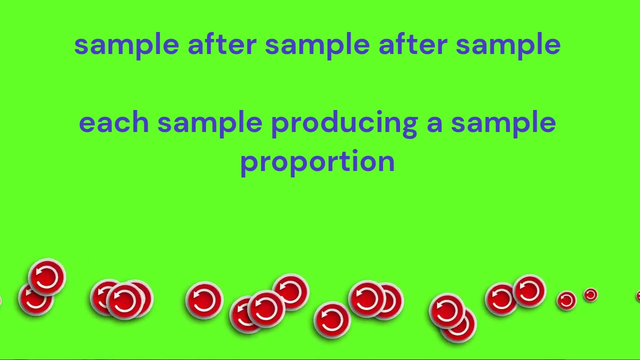 Now if we started to repeatedly sample? take out 230 10 year old kids ask that they believe in the tooth fairy, get a sample proportion and then rinse and repeat like a million times. I mean, if you think about it, there's millions of 10 year old kids across the United States. that means that 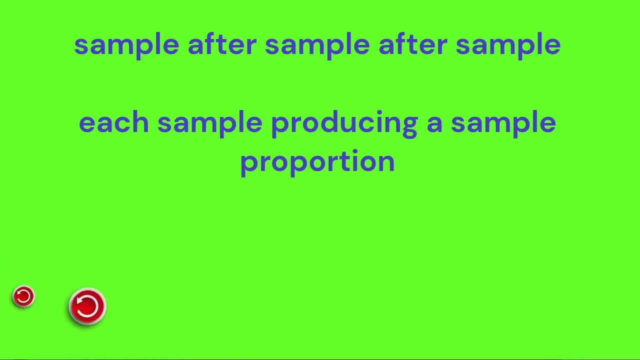 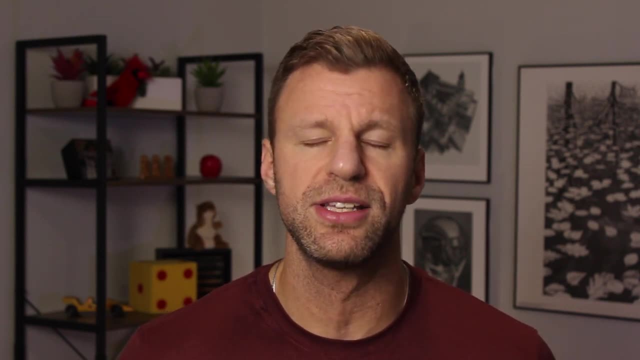 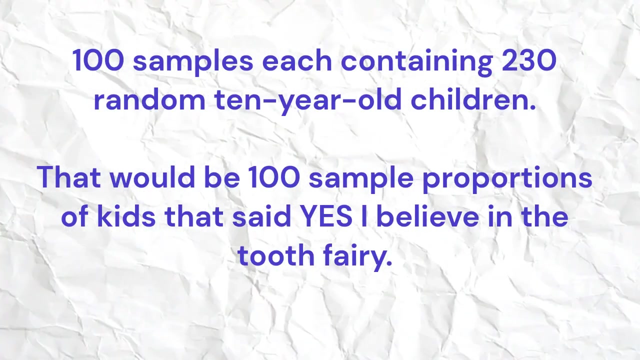 there's probably tons and tons and tons of different samples of 230 of them. So imagine if we just start repeatedly sample 230 kids, 230 kids, 230 kids- we would get a lot of different sample proportions. So for starters, let's just stick with 100.. Let's say that we looked at 100 samples. 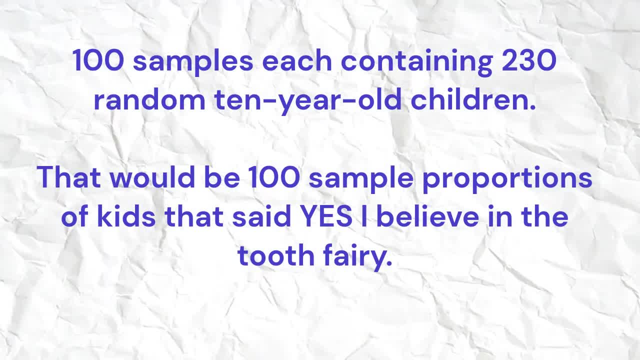 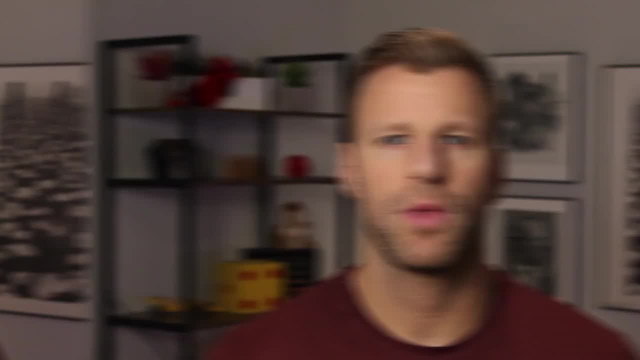 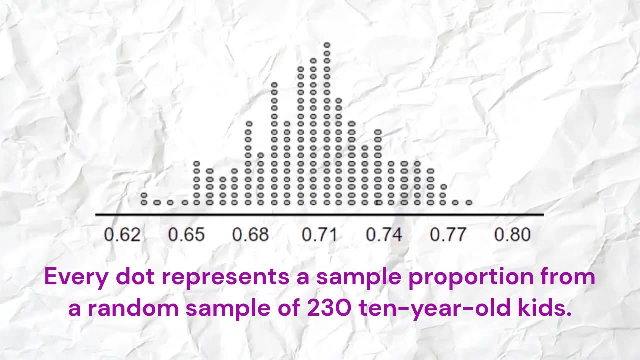 each containing 230 students, 10 year old students- and we asked them: do you believe in the tooth fairy? that means we're going to have 100 sample proportions. Well, here are the results of those 100 samples. Here we see a distribution where every single one of these dots represents the 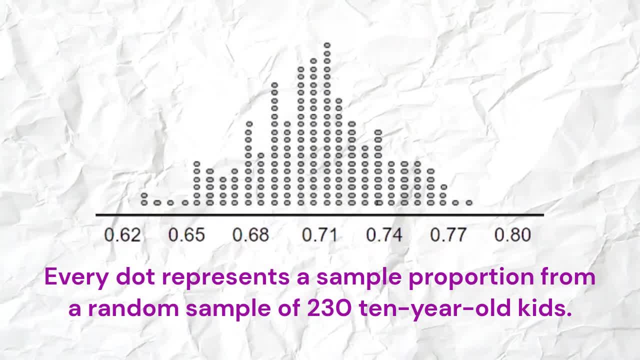 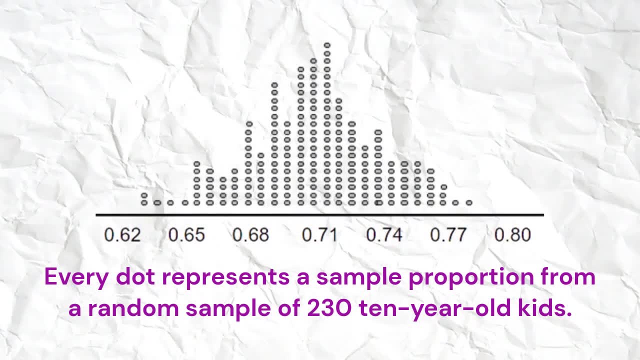 sample proportion from a sample of 230 random 10 year old students and it's showing us the sample proportion of those students. So we're going to take a look at that and we're going to take a look at those kids that said they believe in the tooth fairy. So we see a dot for every one of. 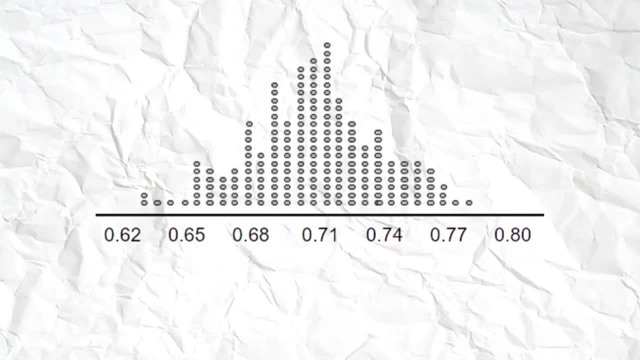 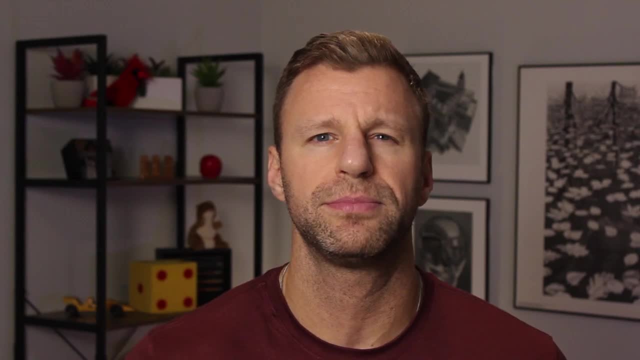 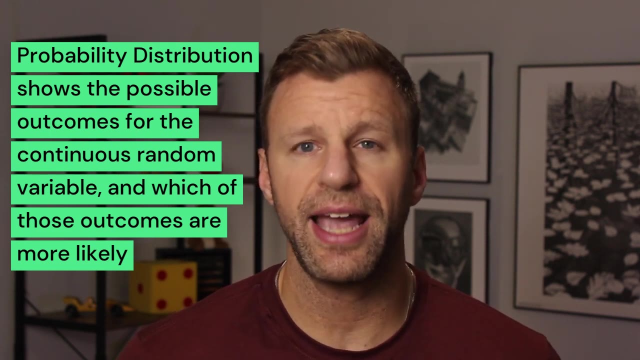 those samples We see: some low is around 63 percent, some as high as 78 percent, but most are right around 70, 71, 72 percent. This is what we call a probability distribution. It shows the values of the continuous random variable, In this case the proportion of 10 year old kids in a sample of 230. 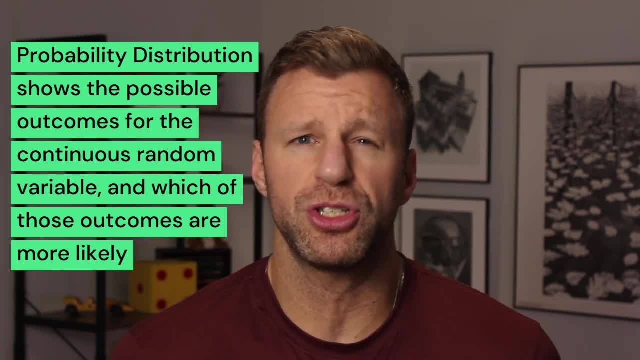 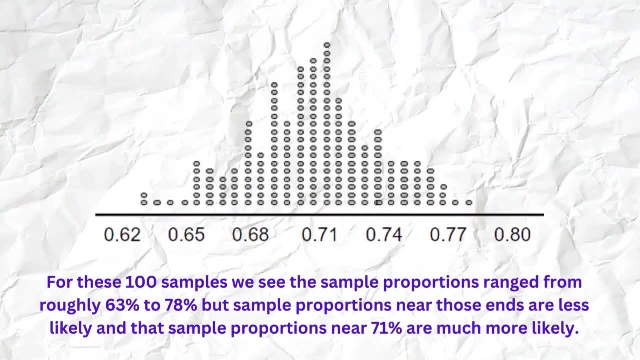 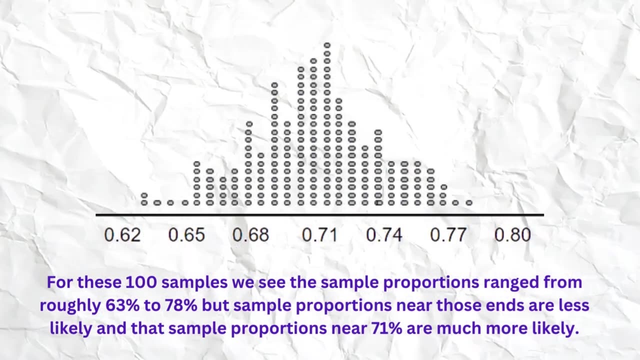 that believe in the tooth fairy, and it shows what those sample proportions could be, As well as which ones are more likely. So for these 100 samples we see that it ranged from about 63 to 78 percent, but we see that sample proportions down at those ends are much less likely: around 63. 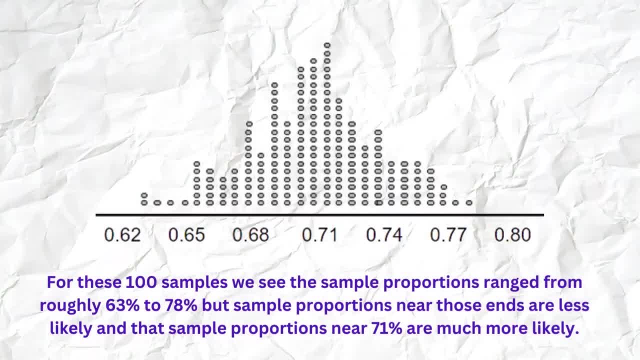 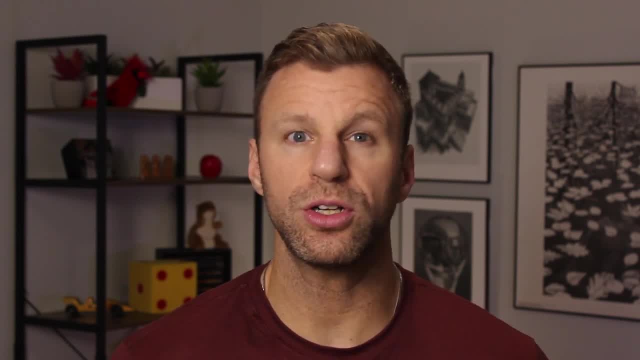 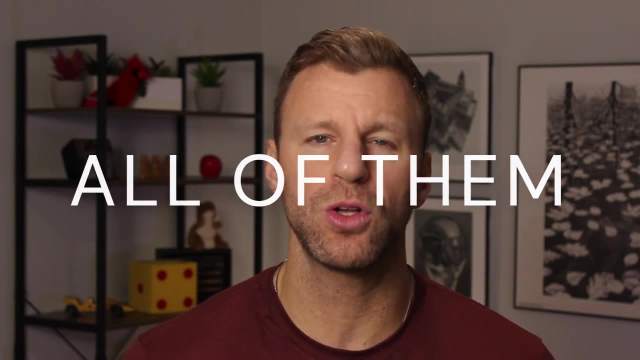 and 78 percent, and sample portions in the middle, around 71 percent, are much more likely. Now imagine, instead of just looking at 100 samples, we looked at all of them, every single possible sample proportion. So what we want to do here is to create a sample distribution of all of those sample. 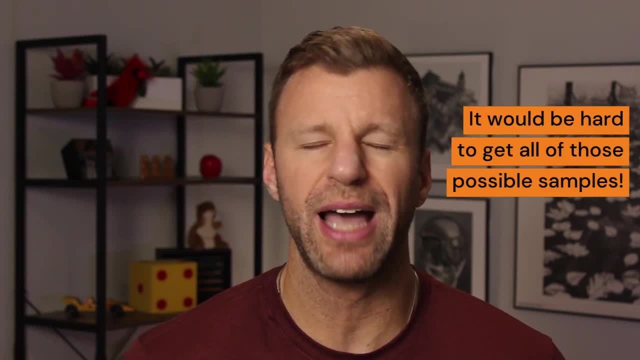 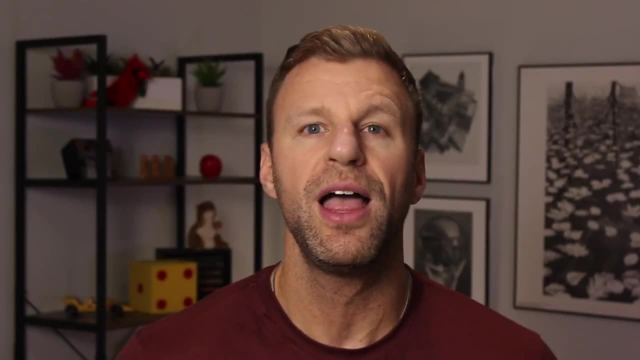 proportions. What we want to do is to create a sample distribution of all of those sample proportions. Well, first, theoretically this would kind of be impossible. but if we could do it, it would be called a sampling distribution for the sample proportions. That's what a sampling distribution is. It's a 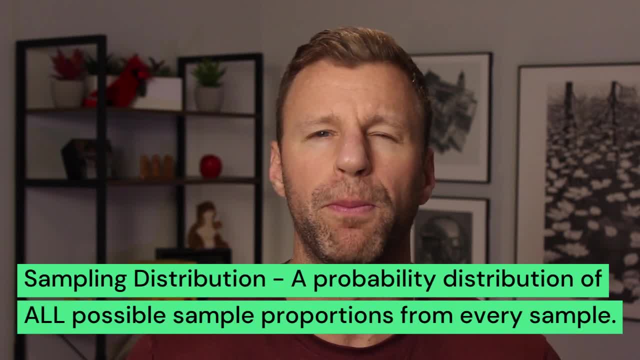 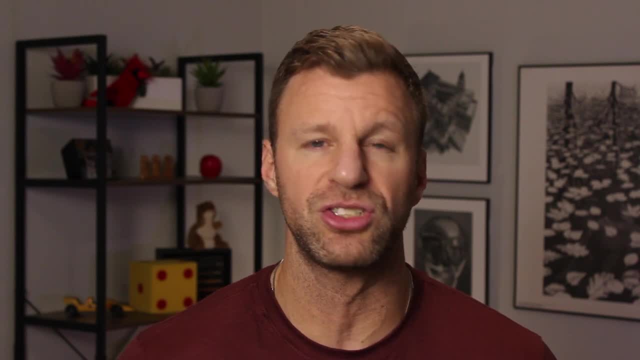 representation of every possible sample proportion from every possible sample of size 230.. Now again, that would be pretty hard to do. So we're going to take a look at that sample distribution and we're to actually look at all those samples. but theoretically we could think about. 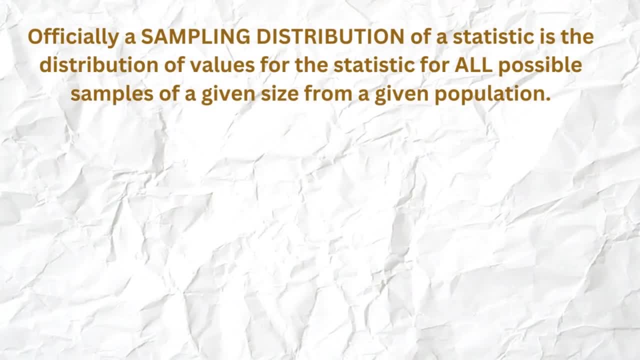 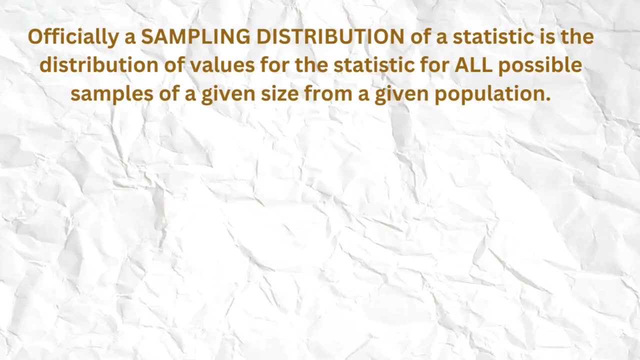 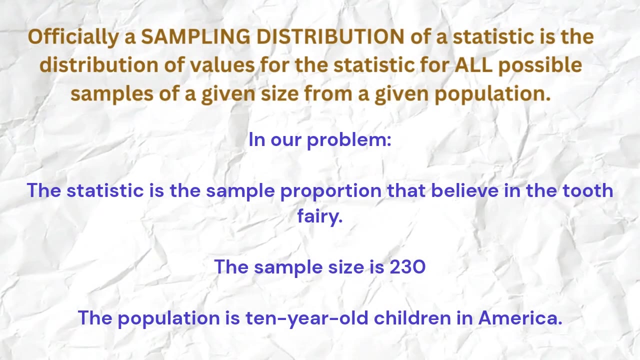 that sampling distribution- Officially a sampling distribution of a statistic- is the distribution of values for the statistic for all possible samples of a given size from a given population. In our problem, the statistic is the sample proportion that believe in the tooth fairy. 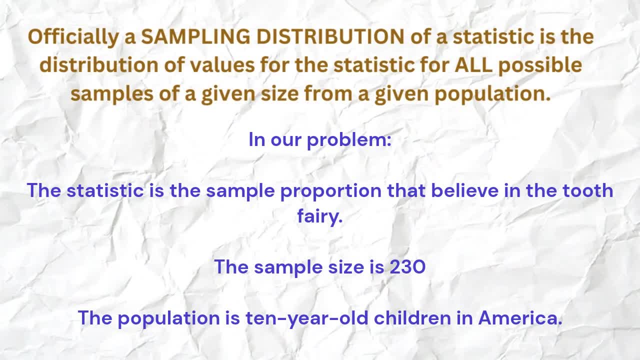 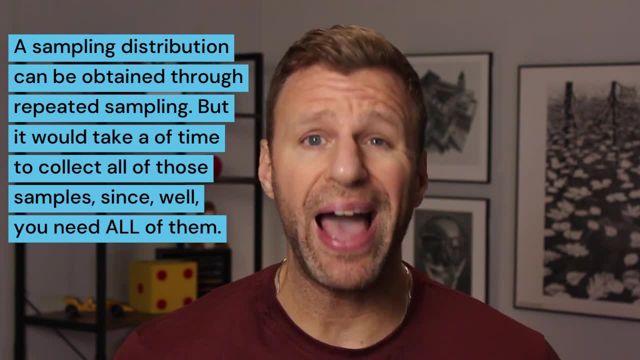 the sample size is two and 30, and the population is 10-year-old children in America. Now, a true sampling distribution can be obtained through repeated sampling. Now, actually taking that many samples would be pretty difficult. but here's the crazy thing. 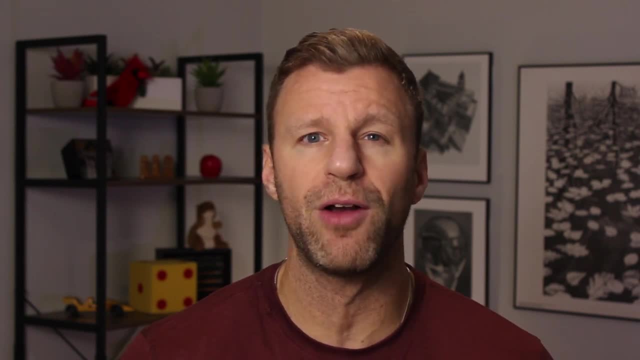 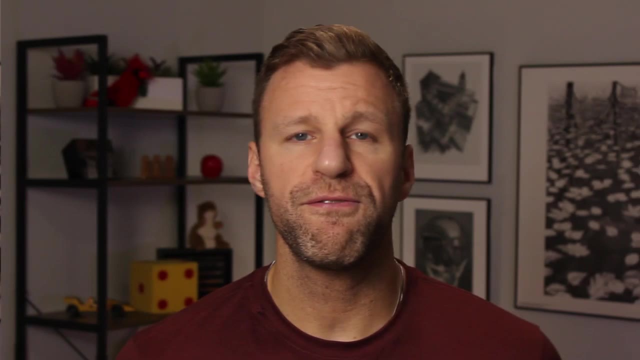 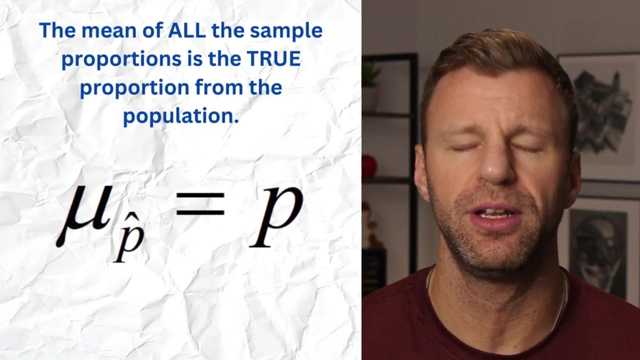 Sampling distributions for sample proportions are very, very predictable. So here are three things we know that are true for every sampling distribution for sample proportions. First, the mean of all the sample proportions will be the true population proportion. Think about that for one. second. 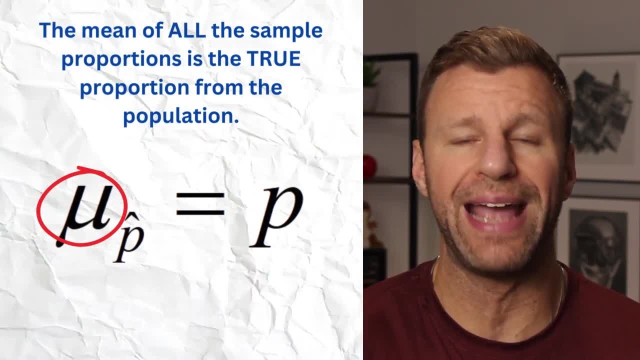 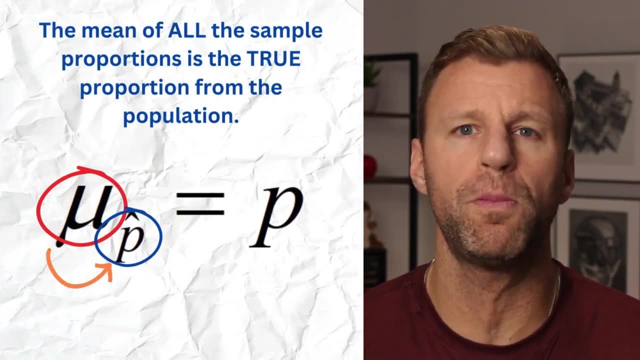 If we took the mean mu of all possible p-hats- remember there's tons of them out there- the mean of all the sample proportions would be equal to the true population proportion, smack dab in the middle. That should make complete sense. 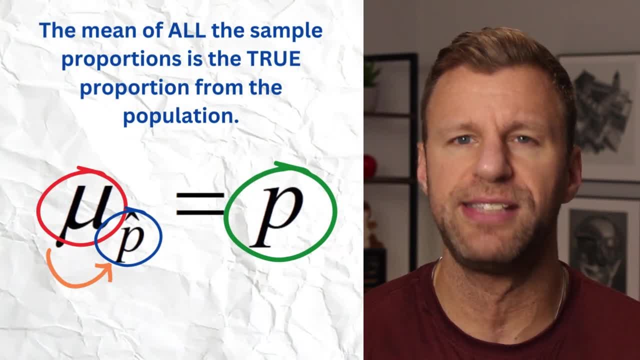 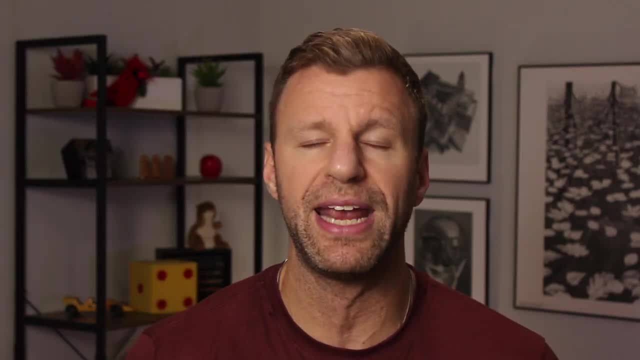 Remember, we expect to get 71% of kids in our sample that believe in tooth fairy. but we know we might not get it, but we expect it to be 71%. That's because the mean of all p-hats should be 71%. 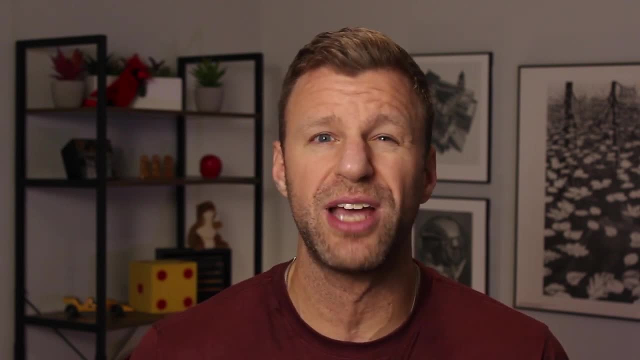 Yeah, some of them are gonna be more than 71%, some of them are gonna be less than 71%, but if we take the mean of them all, we should get that true population parameter right, smack dab in the center. The second big thing we know. 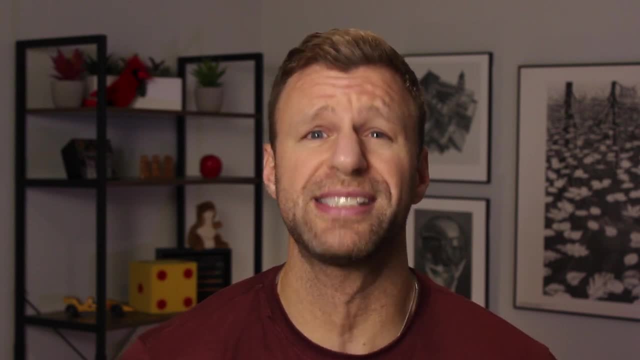 is that sampling distributions are filled with sample proportions and sampling proportions are going to vary And we can actually measure that variation with the standard deviation. So there is a formula for the standard deviation of all those p-hats. It's pretty simple formula. 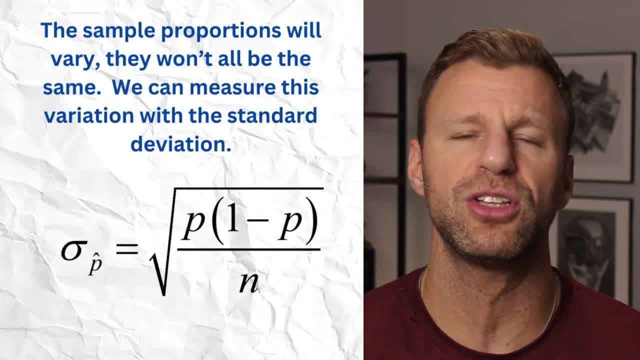 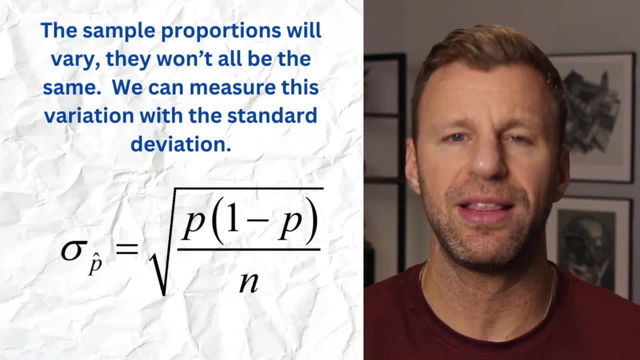 It's a giant square. It's a square root. Inside of that square root is a fraction. The numerator is p, the population proportion times one minus p. that would just be the opposite of p divided by the sample size n. 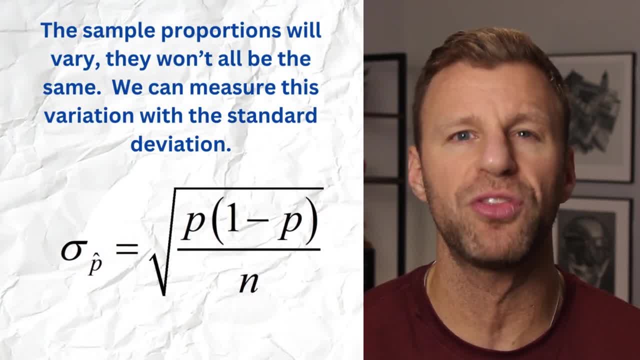 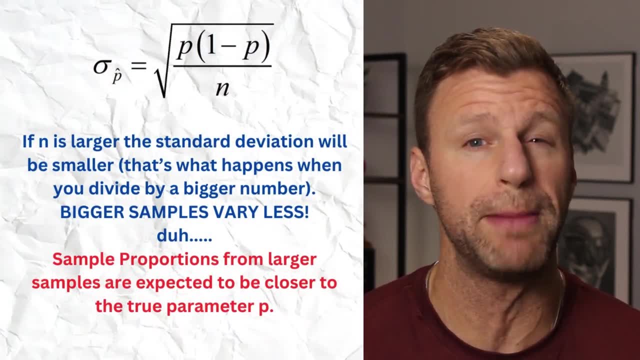 Now, because the n is in the denominator. that tells us that the bigger the samples we select, the lower the standard deviation, And that should actually make complete sense, because bigger samples should be more accurate And if bigger samples are more accurate, that means that they're going to vary less. 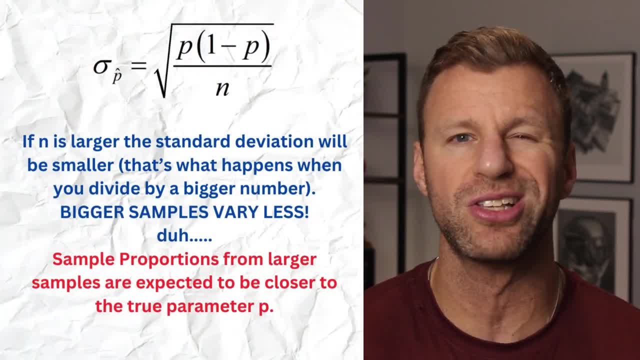 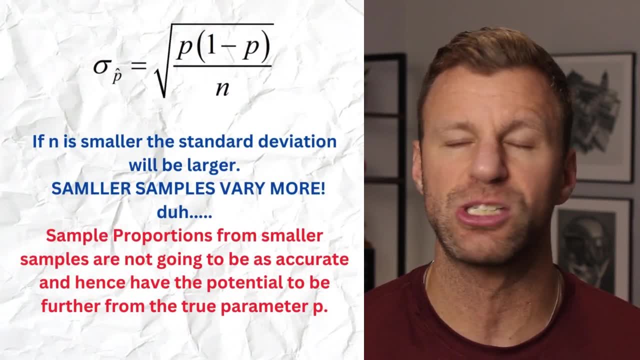 And that means that we would get a value for our sample proportion that's closer to the truth. Smaller samples are going to vary more. A smaller sample could be all over the place, and that's why they would produce a larger standard deviation. 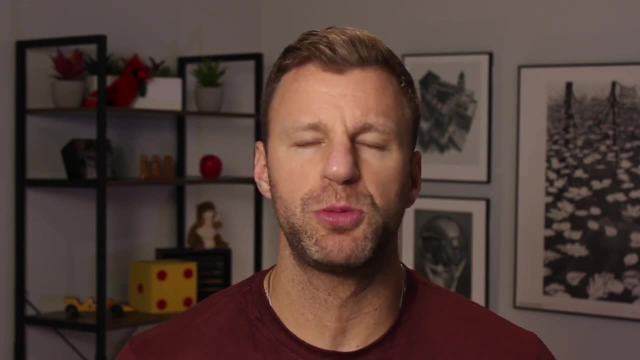 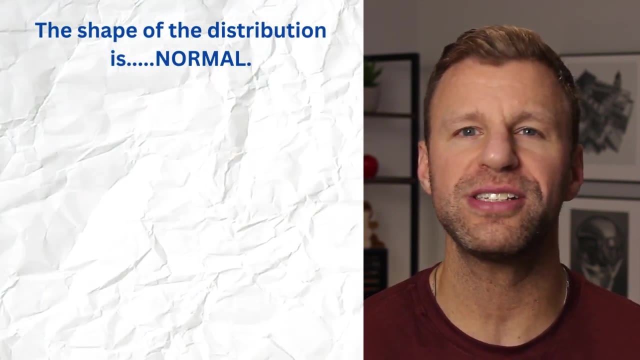 The third feature that we know is true for all sampling distributions, for sample proportions, is that the shape of the distribution is going to be normal. Now, this is awesome because, well, we love the normal model. but hold on a minute. Here comes the third rule. 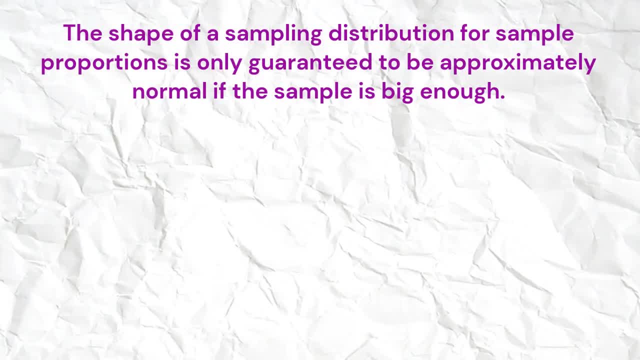 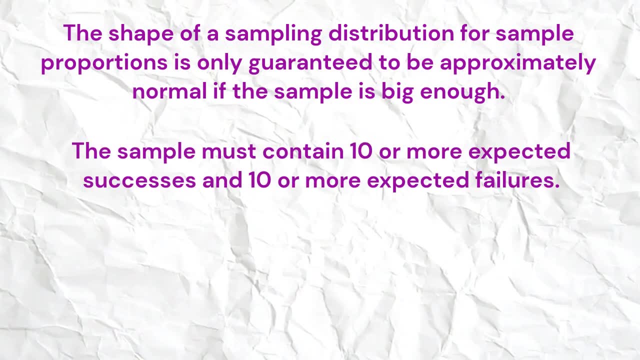 The shape will only be normal if our sample is big enough. Well, how do you know if your sample's big enough? Well, it's actually a pretty simple rule. We simply have to have 10 or more expected successes and 10 or more expected failures. 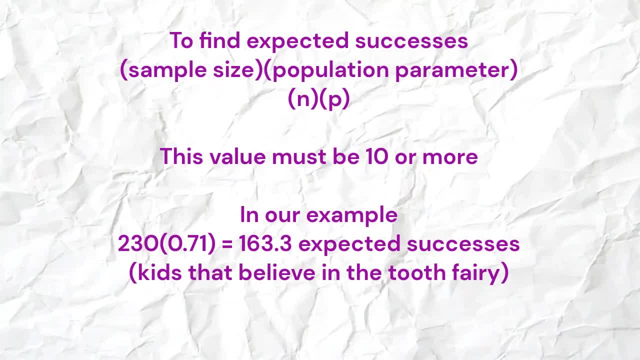 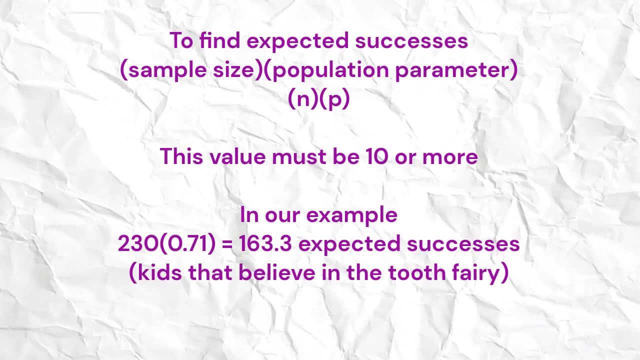 So how do you check if you have that? Well, you simply take your sample size n and you multiply it by p. That would be your expected number of successes. As long as that number is 10 or more, we're good to go. 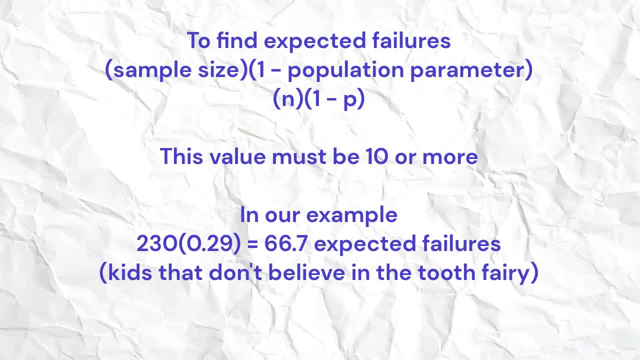 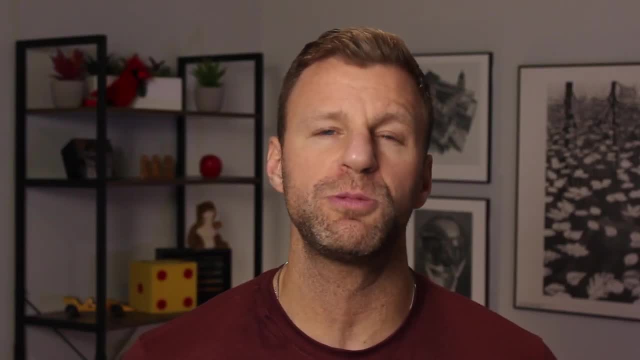 Then we take our sample size 230 and multiply it by 1 minus p. this is going to produce our expected number of failures, and this number needs to be 10 or more as well. So as long as we have 10 or more expected successes and failures in our sample, then we are 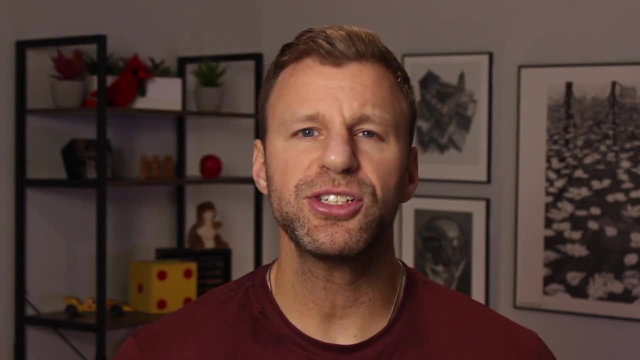 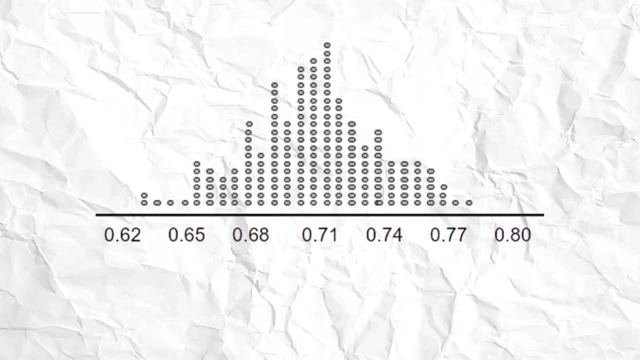 big enough for that shape to be normal. Now let's go back to that distribution that we had for 100 samples. Now, by no means is this a true sampling distribution, because a true sampling distribution has the results for every possible sample proportion out there. Well, this was only looking. 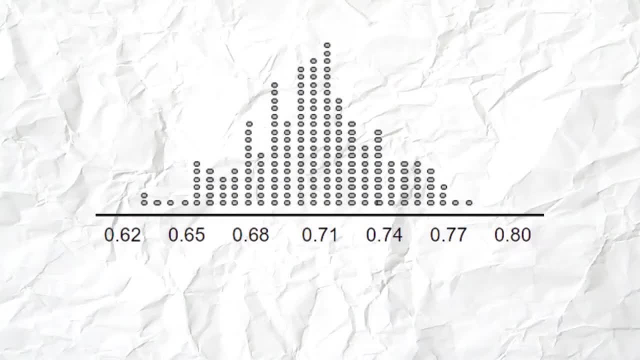 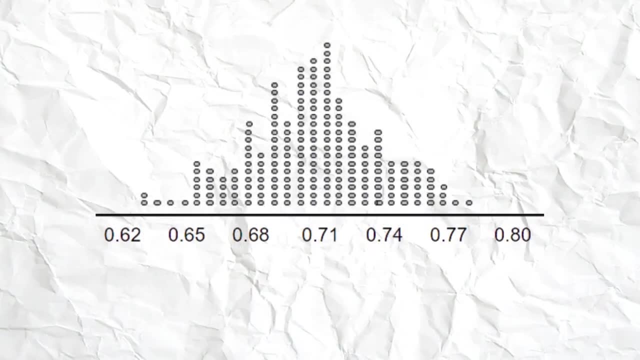 at 100. so it's like the start of a sampling distribution. But what I want to show you is that those three qualities that I just spoke about are visible in this graph. First, we already see the center. the mean of all the sample proportions is right around 71 percent, which is what the true 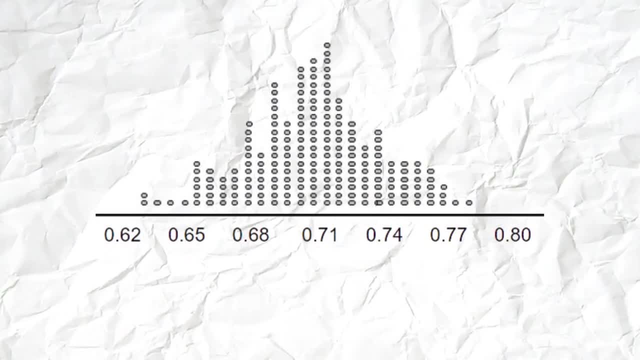 population proportion is. We also see the fact that there is a standard deviation, because samples do vary. Some samples are more than 71 percent and some samples are less than 71 percent, And the last thing we see is the shape. It actually does not change. It does not change, It does not change. 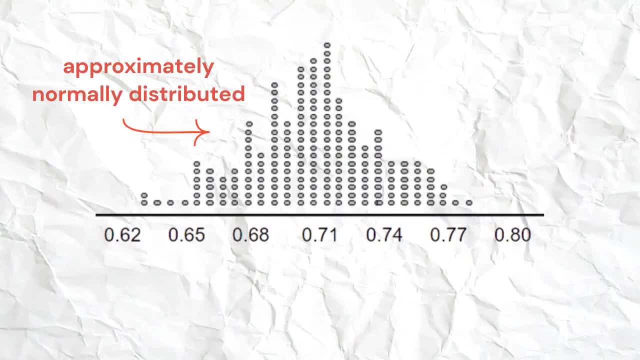 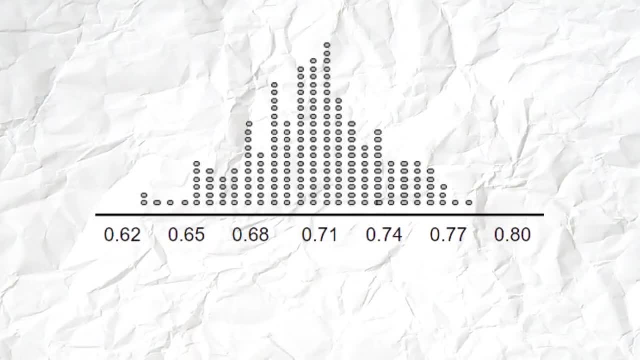 It does look roughly normal. where we see on the tails, the far left and the far right are way less likely outcomes than the outcomes in the middle, which are right around that 71 percent. So we do kind of see this nice mound shape, normal distribution forming, and we've only looked at 100. 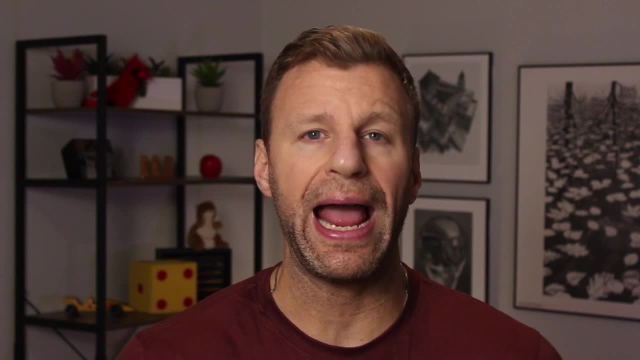 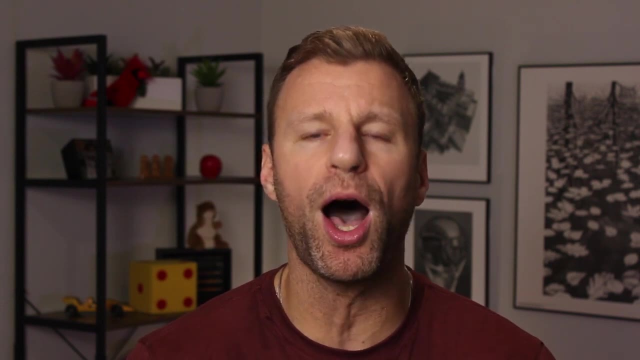 samples. Now again, it's very difficult to create an actual sampling distribution because it's very hard to look at every possible sample. But what we can do is we can model a sampling distribution and this is the most important part of the distribution. So we can model a sampling distribution. 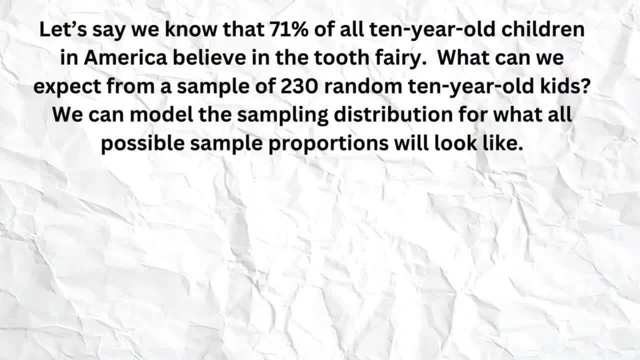 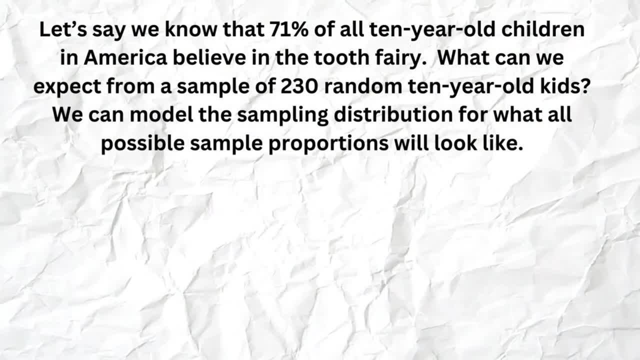 and this is the most important part of the video. So let's just say that 71 percent of kids 10 year olds across the United States believe in the tooth fairy. What would we expect for a sample of 230?? Well, we don't even actually have to go and get any samples to know what that sampling 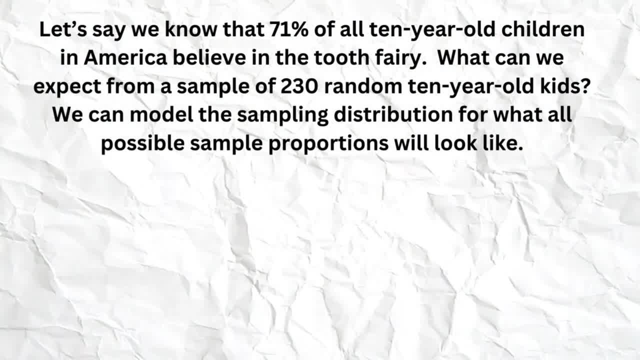 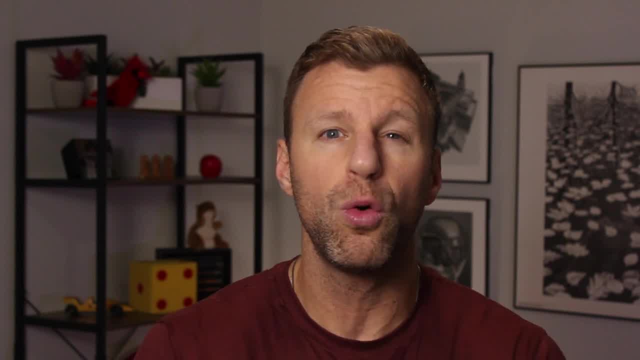 distribution could look like. Now that's crazy. Let me repeat that one more time: As long as we know the sample size- 230- and we know the true population proportion- p 71 percent- we don't have to look at any samples to know what that sampling distribution could look like. So we don't have to. 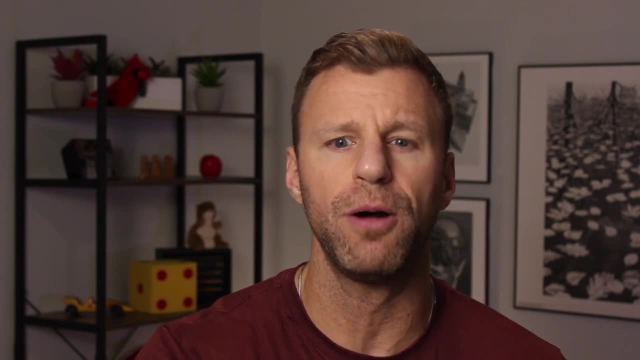 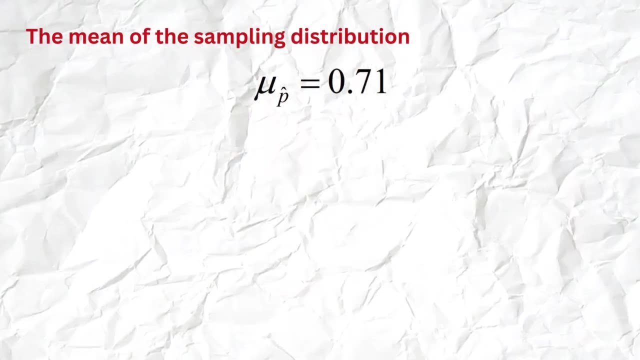 know what the sampling distribution will look like. Here we go. First, the mean of the sampling distribution will be the mean of all the p hats, and that should be the truth, Right smack dab in the center: 0.71.. But again, the rule is that those samples do have to be random to avoid bias. 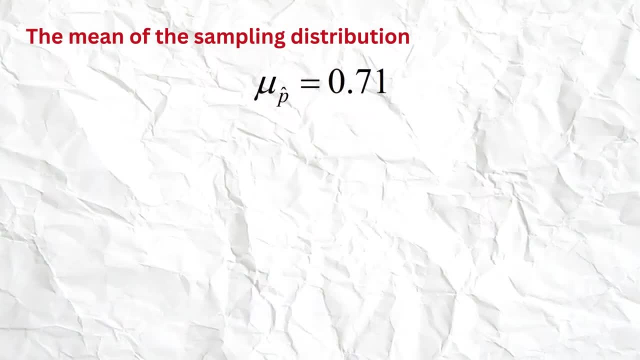 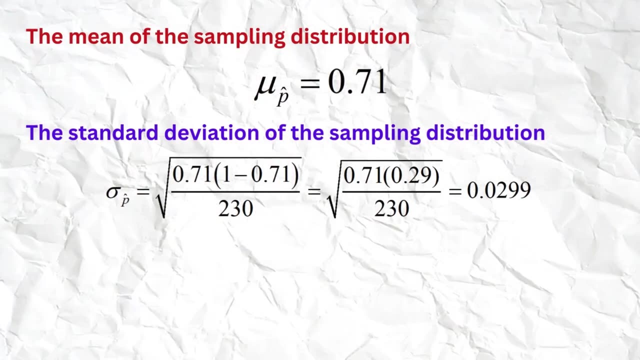 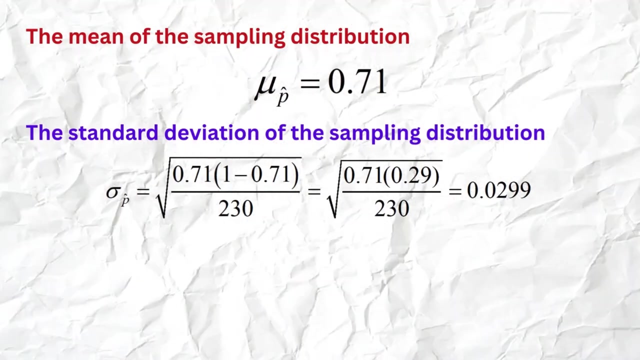 Next up, we have the idea that those sample proportions are going to vary. So the standard deviation of those sample proportions, p hat, is going to be the giant square root of 0.71.. That was our p times 1 minus 0.71, which is going to end up being 0.29 divided by 230, and we get. 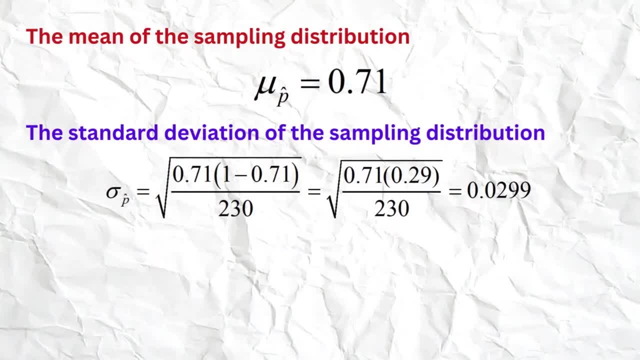 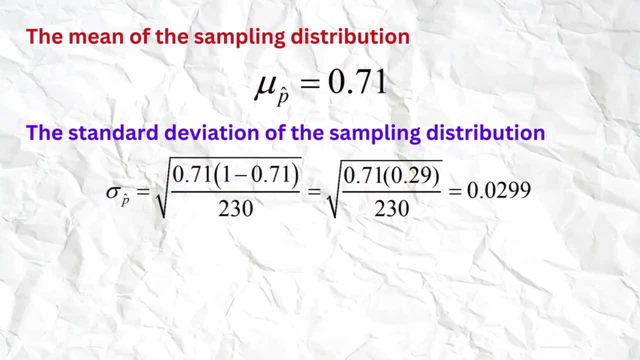 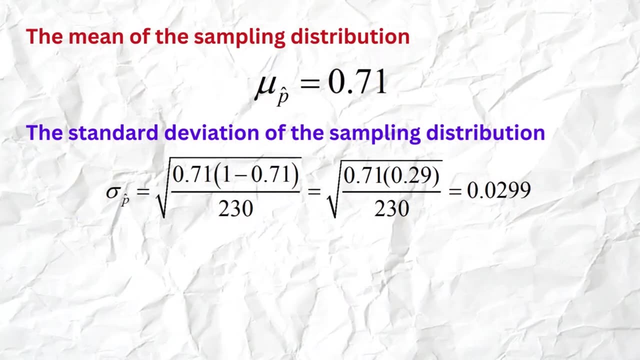 0.0299, like just short of 3 percent. But again, the only way that this formula is usable if we know that we have independence between all of our samples, Which if we don't replace, remember, we actually don't have independence. But as long as our sample size of 230 is under 10 percent of the 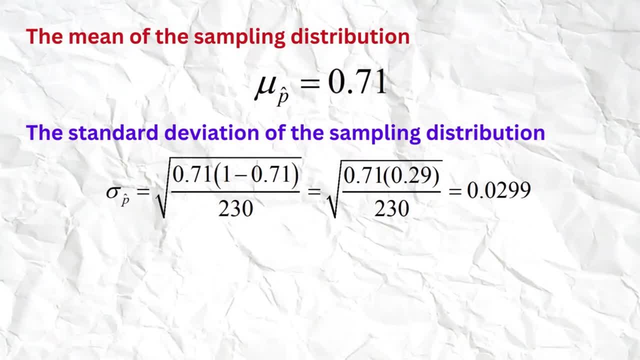 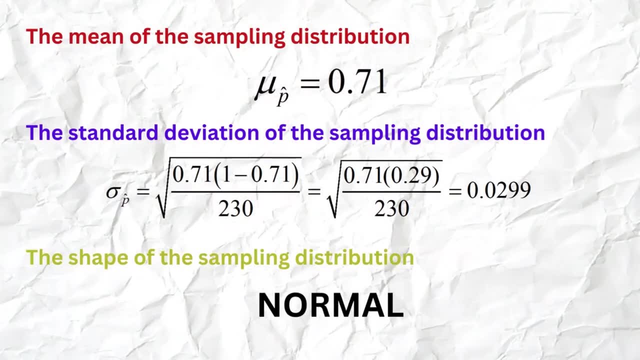 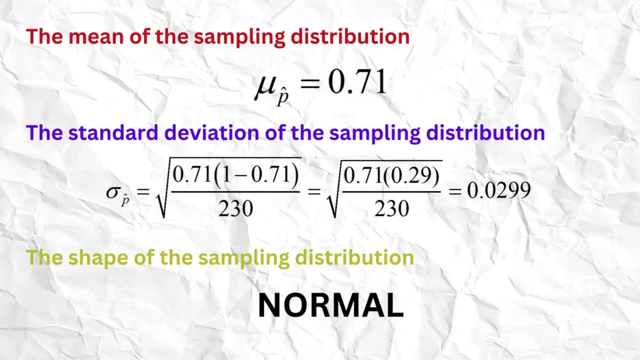 population, it's totally fine to assume that they will be independent, even though we don't have enough sample size. So we simply have to take 230 times 0.71 and 230 times 0.29.. As long as our successes and failures are both 10 or more- which they are- then the sampling distribution will be. 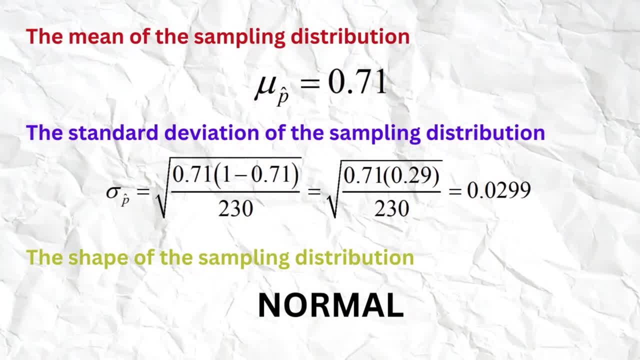 normal. So here is a picture of that sampling distribution And let me remind you for a third time, we haven't actually officially looked at any samples and we already know what they would be. So here is a picture of that sampling distribution and let me remind you for a third time, we haven't actually officially looked at any samples and we already know what they would be. 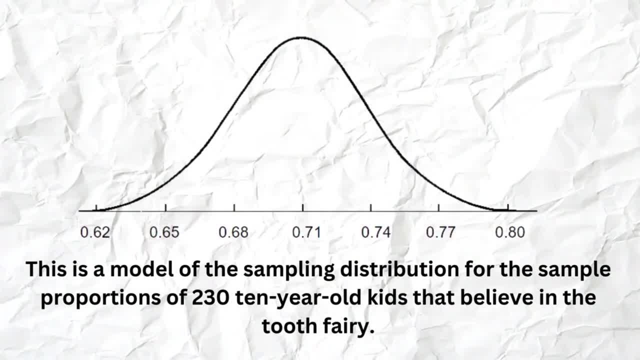 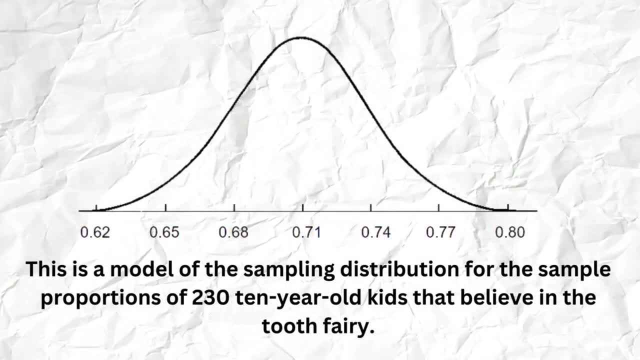 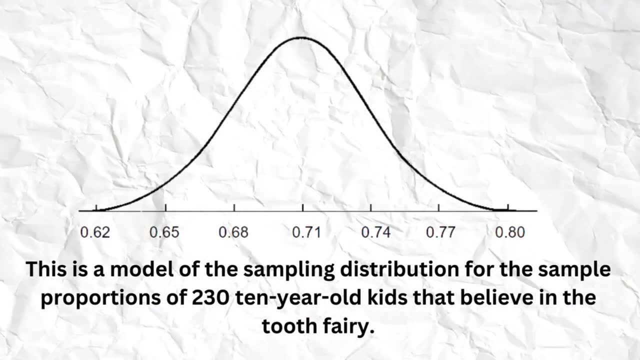 will all look like, or at least we can model what they'll all look like. so right smack dab in the center, we see the mean of 0.71. then i went up one, two, three standard deviations. now remember our standard deviation was 0.0299, which is really really close to three percent. so i went up to 74. 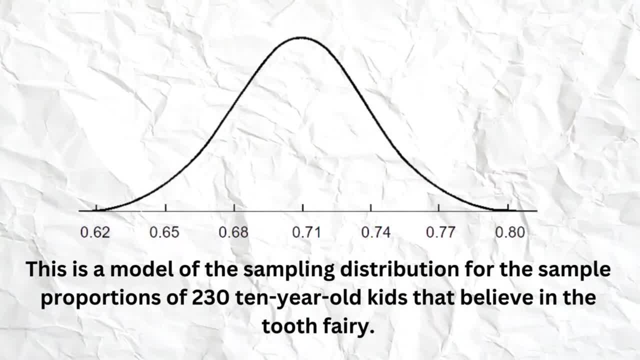 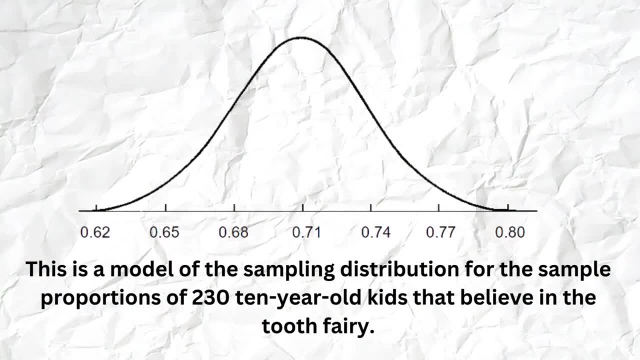 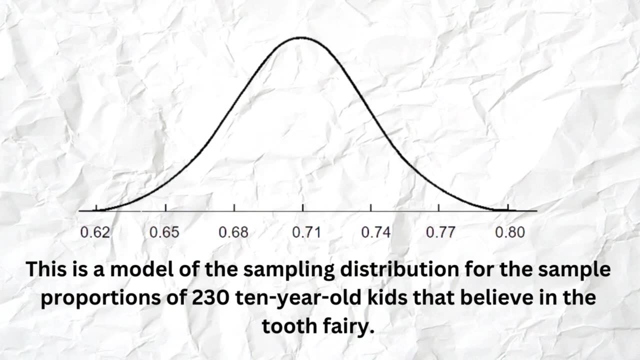 percent, seventy seven percent, eighty percent. then we're going to go down one, two, three center deviations: 68, 65 and 62 percent, and of course, the last part is that this shape is normal now. so this is what it looks like and again, it's awesome. so before we even go and look at a sample, 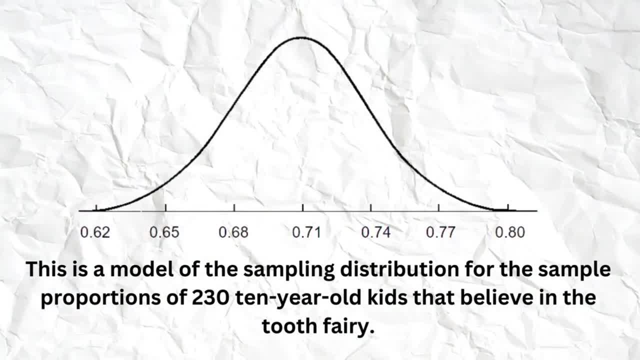 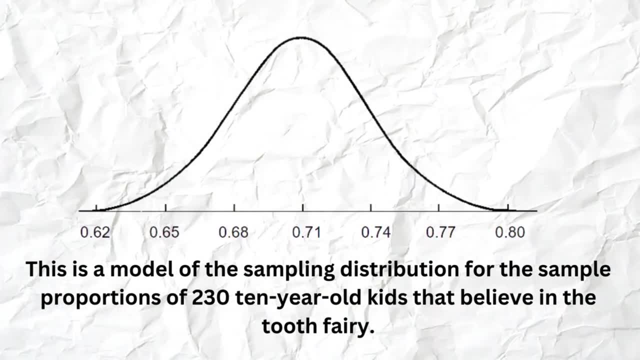 of 230 students, we already know what to expect. we would certainly expect something around 68 to 74, because that's where the large majority of sample proportions will be. a sample proportion of like 90 percent or 50 would be extremely unlikely, probably not going to happen, and that's it. 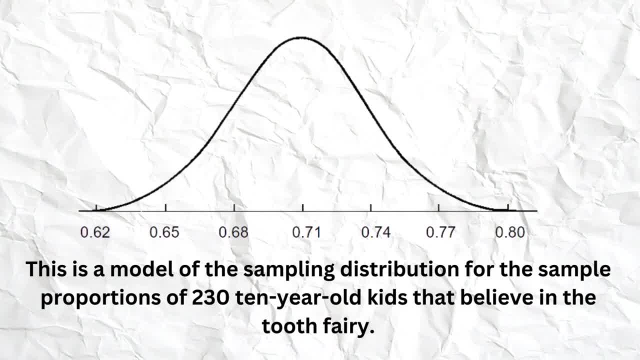 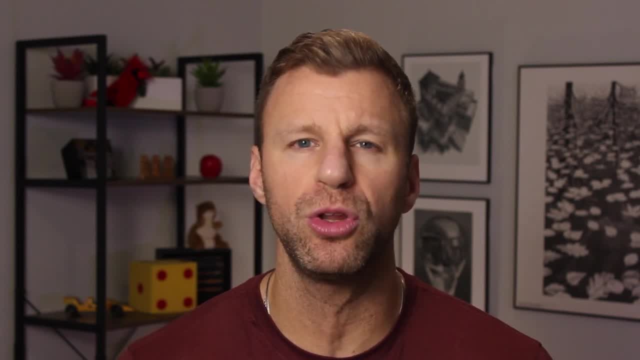 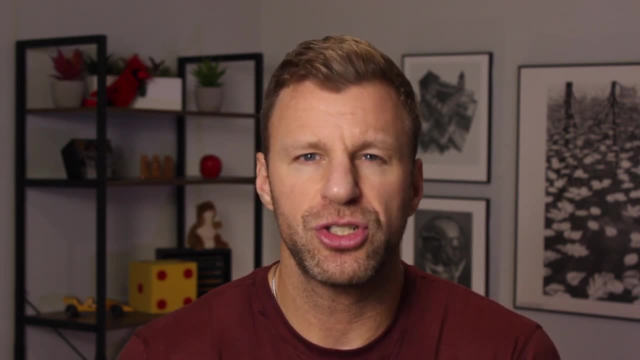 this is how we could build a sampling distribution for sample proportions. what we're doing here is simply modeling what all possible sample proportions would look like of a certain sample size. because, remember, if we change the sample size and we change the standard deviation and that could shrink the model in or spread the model out, and all of those samples do have to be taken from the 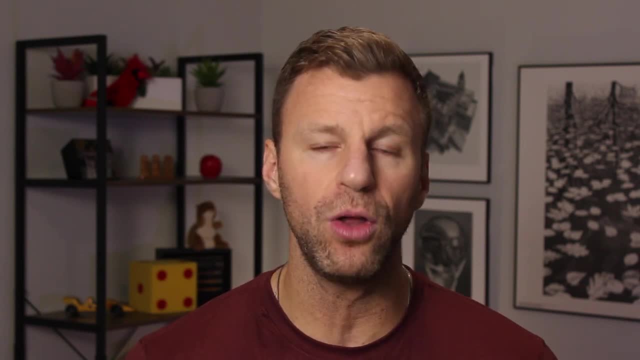 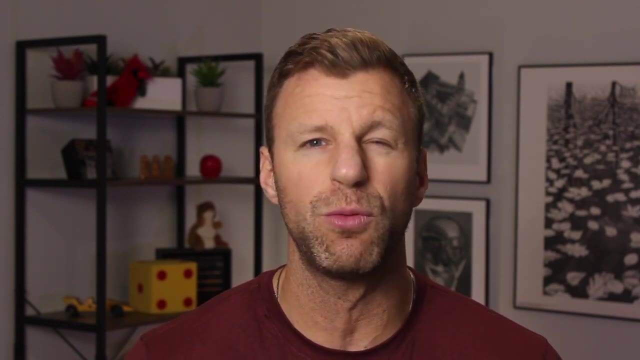 same population. now, once we have this model- it is a probability distribution. it shows us what's most likely in the center and what's less likely out towards the ends. and once we have a probability distribution and it's more likely to be in the center, we're going to be able to get a more likely 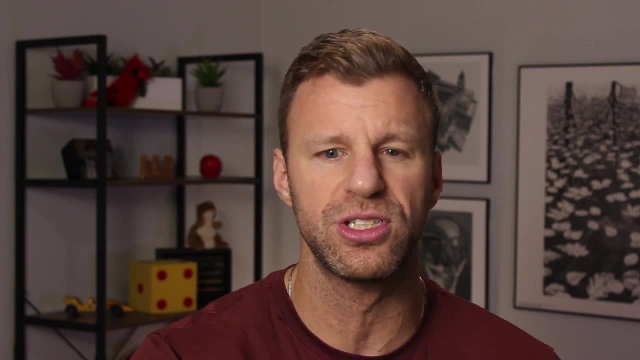 out towards the ends and once we have a probability distribution, we're going to be able to get a more likely out towards the ends and once we have a probability distribution, we're going to be able to get a more likely. we can answer some pretty pretty cool probability questions like this: 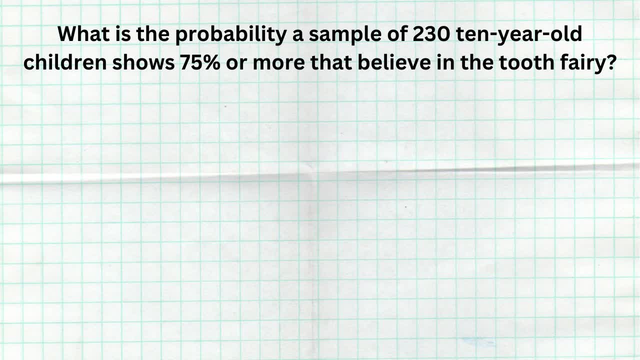 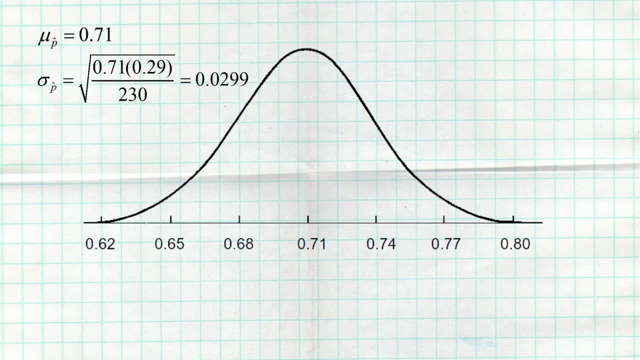 let's say that we want to know what is the probability that a sample of 230 10 year old children shows 75 or more that believe in the tooth fairy. well, all we have to do is figure out: where does 75 fall on our model? well, first we're going to go ahead and look at our model and we see. 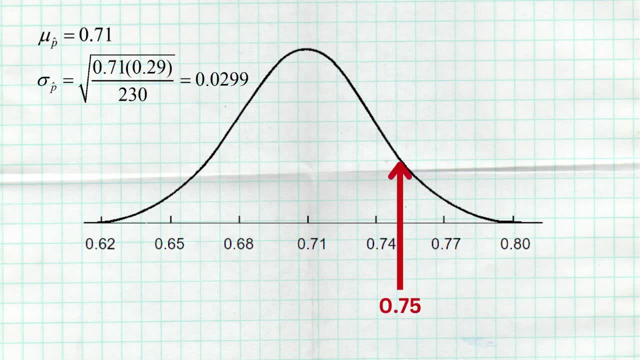 that 75 percent falls a little bit more than one standard deviation above the mean. but if we're going to answer probability questions about it, we need to figure out where it falls on the standard normal model, which means we need z scores. so we're going to go ahead and find the z score for 0.75 by 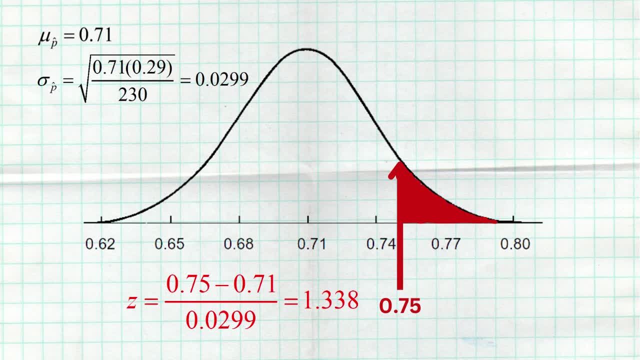 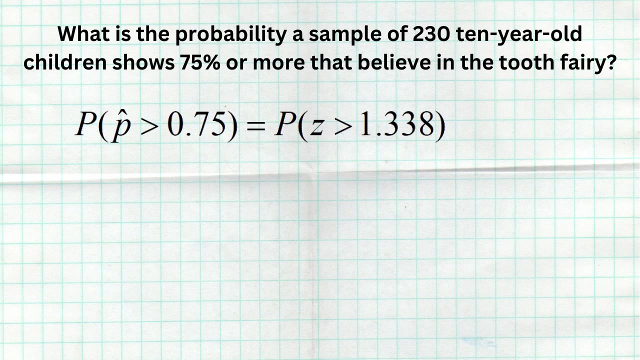 subtracting the mean 0.71, dividing by the standard deviation 0.0299, you guys know to find a z score and we get a z score of 1.338. so we're trying to find the probability that a sample portion is greater than 0.75, which is the probability that a z score on the standard normal model is greater. 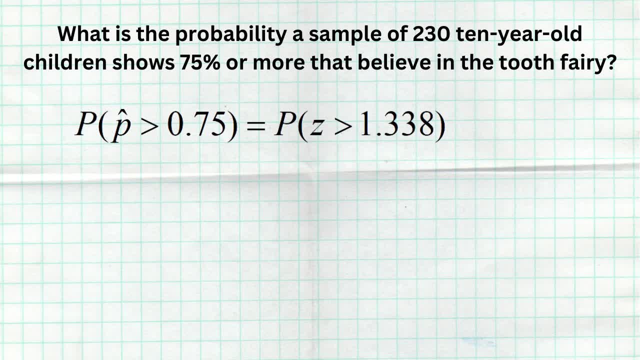 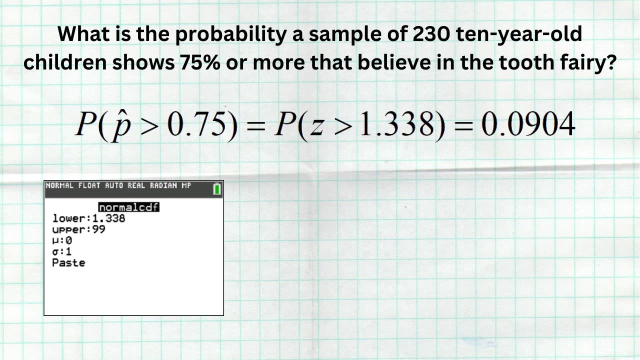 than 1.338. now how are we going to do that? well, of course we could use our calculator or we could use a z table. i'm going to go and use the calculator here. use normal cdf, start at a lower value of 1.338, go to an upper value of 99, acting like infinity, and i get 0.0904. that means 9.04. 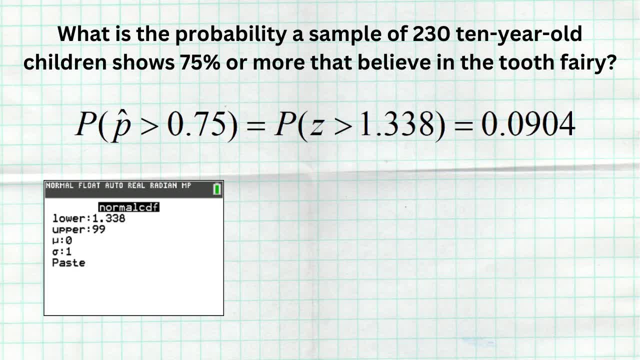 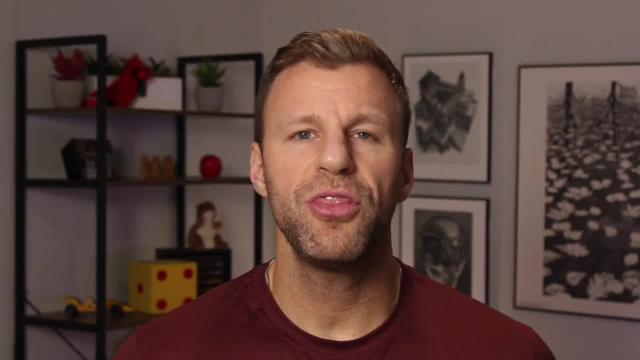 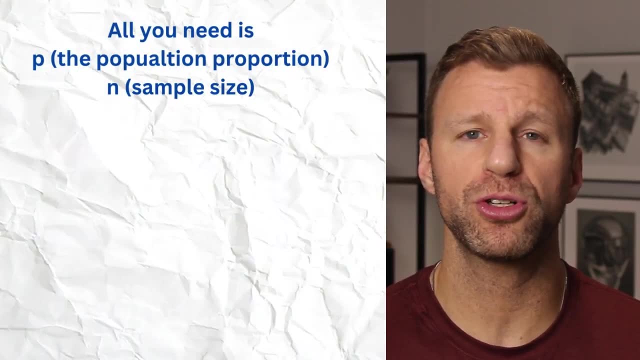 of all possible sample proportions of 230 children, taken from a population of all 10 year olds, will be greater than 75 percent. that's how easy it is to build a sampling distribution for sample proportions. all you need is two things: the population proportion, p, and the sample size n. that's it. then you could 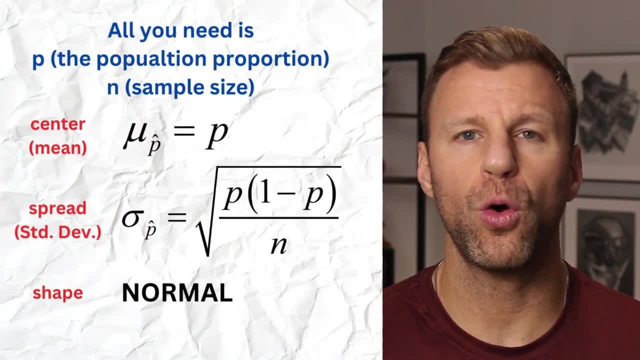 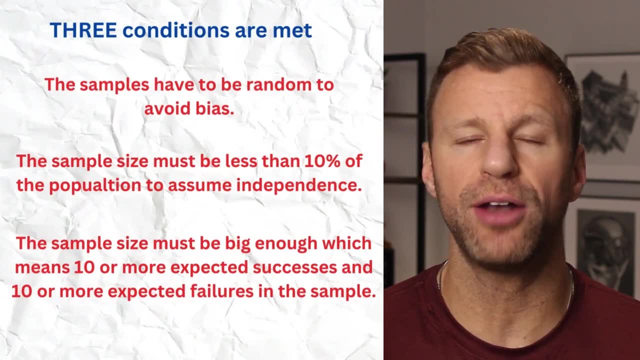 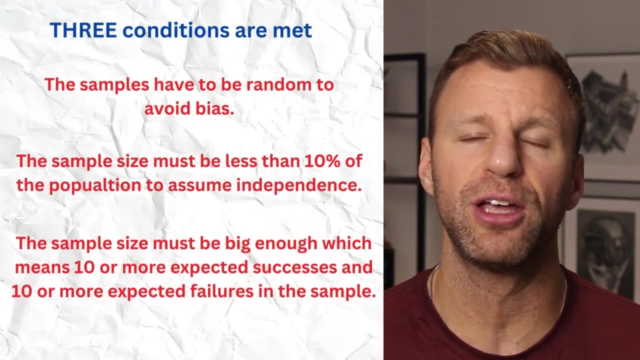 find your mean, your standard deviation and, of course, the shape. but don't forget about the three rules. the sample's got to be random, the sample size has to be under 10 percent of the population and your sample must have 10 or more expected successes and 10 or more expected failures. to 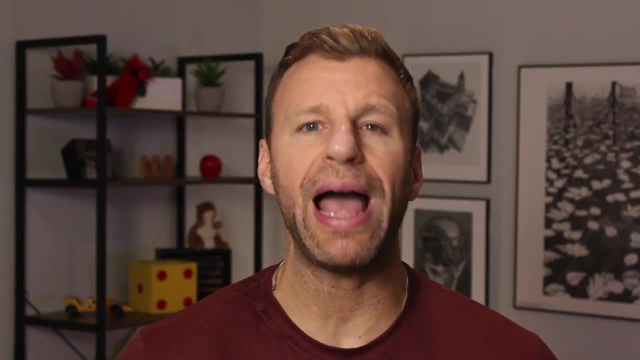 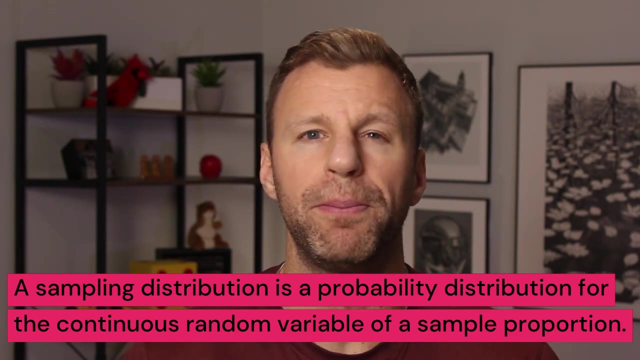 do good in order to get the sample size right. if it's a sample size, there's a snake here and it's a lot easier than the standard average distribution, and this is where we need to be careful, because it's really not going to work just to get all these numbers right.